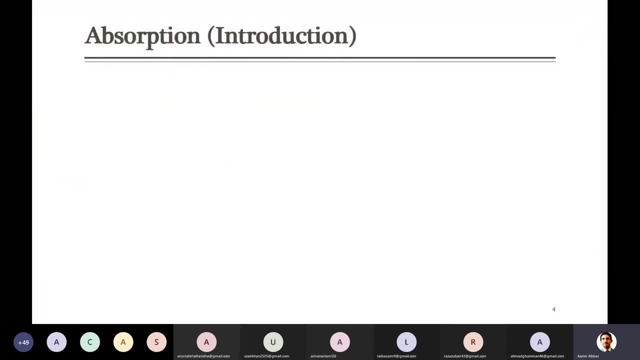 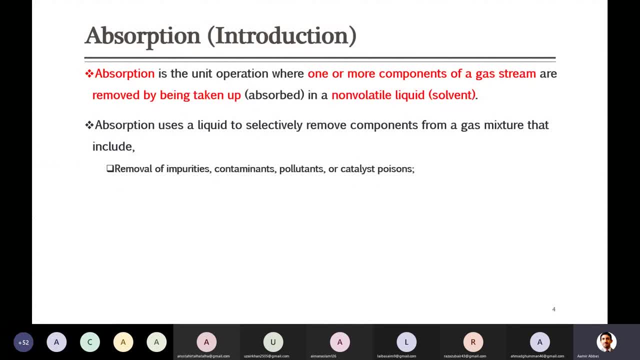 So what is absorption Then? the other purpose of this absorption sometimes can be recovery of valuable chemicals. So it's mean it is not necessary that always we remove some of the contaminants or impurities with the help of absorption. Sometimes maybe you will be absorbing those things which are valuable and all other gas will not be useful for you. So here the example is same, that's, for example, CO2 removal from natural gas. 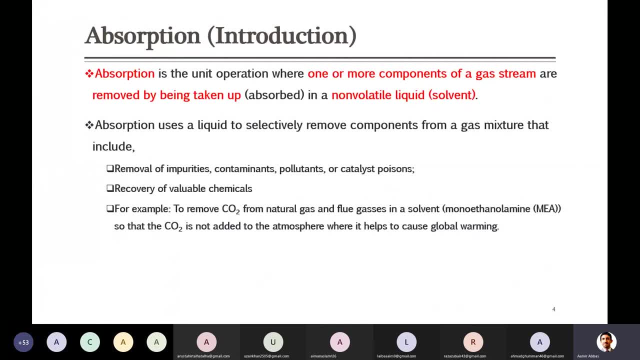 So what is absorption? So what is absorption? So what is absorption? So here the example is same. that's, for example, CO2 removal from natural gas. So what is absorption? removing co2, it's mean this is one of the pollutant that should not be added to the 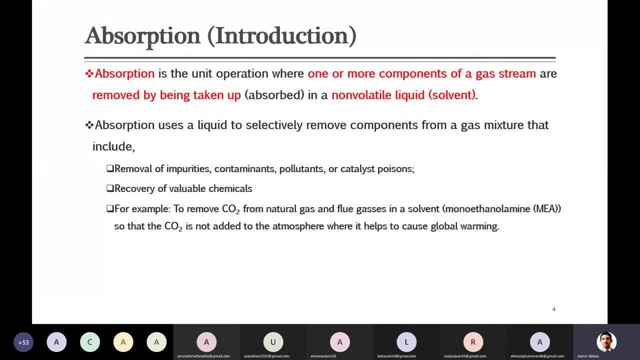 atmosphere. due to this reason, we used to remove co2 from, by the way, flu gases, but from natural gases. co2 will remove on the production sites. if you don't remove co2 from the natural gas, you will need or you have to put extra cost by pumping the co2 along with natural gas. 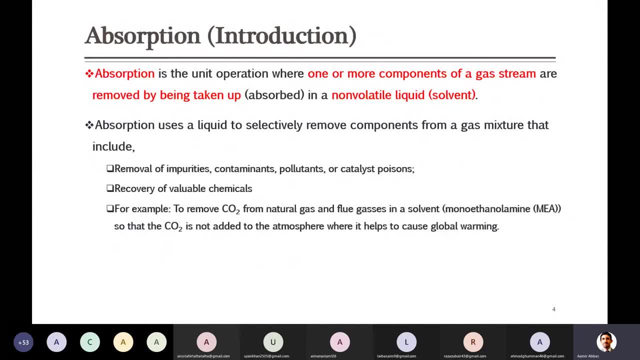 along with the pumping cost, it will be occupying some volume inside the pipeline. so, due to these reasons, it is necessary that co2 should be removed from natural gas, uh, so that you don't have to put extra cost on its pumping as well, as like it will be occupying some volume and at that time 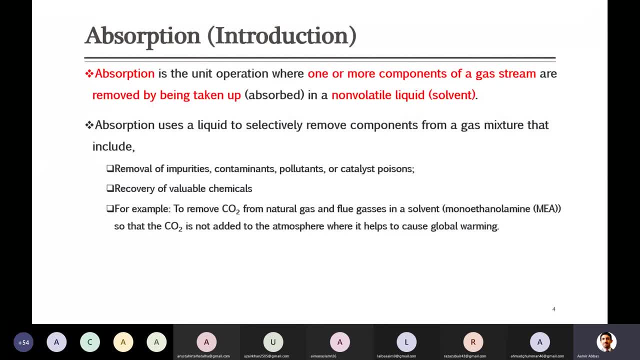 uh mean wherever you are burning the natural gas. it will not provide you any value. so whenever you are using this technique of absorption, uh mean the species of interest. species of interest mean those species which we are absorbing. that may include all components present in the gas. it's. 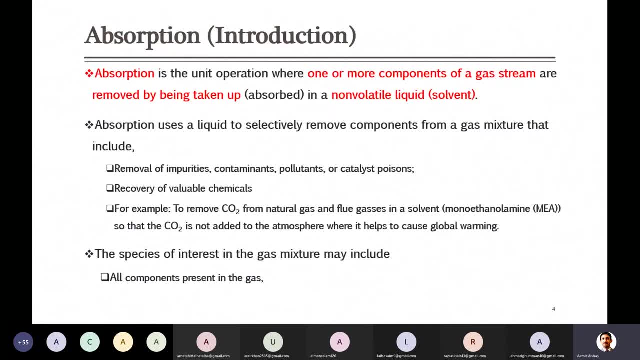 mean the component which we are absorbing. that can be of some benefit, as well as all those component of the gas that are not absorbed. they can also be of some interest to us. so only the component that are not absorbed. sometimes your component of interest are those which are not absorbed, for example, in this case. 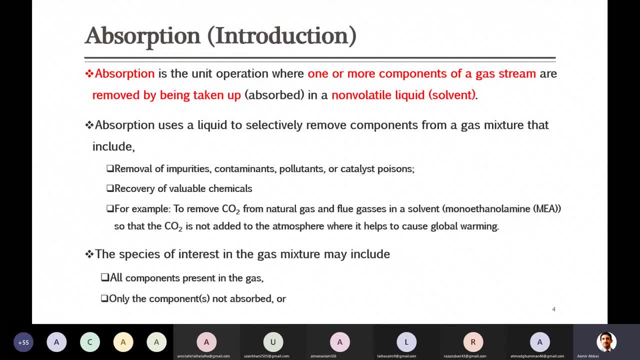 of removal of carbon dioxide from natural gas. i mean, when we have removed co2, uh, all other gas it will be leaving from the system. that is, i mean, of our interest, because that is used for the burning purpose, and then only the components which are absorbed, uh mean they, they can be of benefit. that 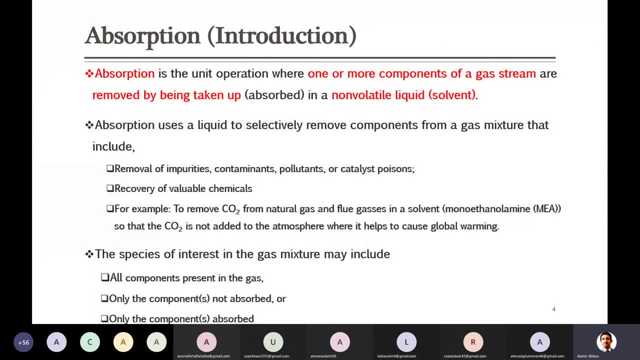 components which are only absorbed. so it depends on your application: either the thing which is absorbed that is of benefit, either which is not absorbed of the benefit, or sometimes both of the gases can be of your benefit. uh, because we use this technique a lot in the industry. so, uh, some, most of the time, when you are using these, 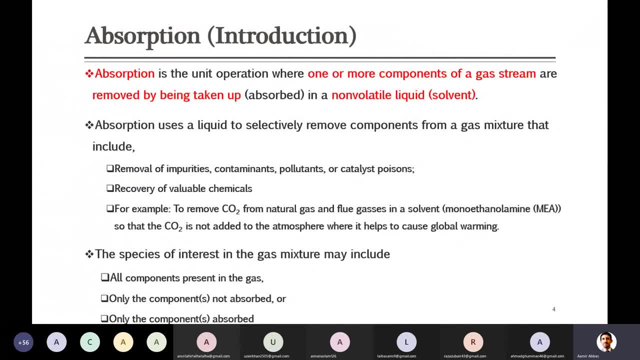 techniques in industries. uh, maybe the gases which you are capturing, they are also being used in some next operation as well as- which are not absorbed- we are also using some next operation as well as- which are not absorbed are not mean captured, they can be of the same. so all those species which are 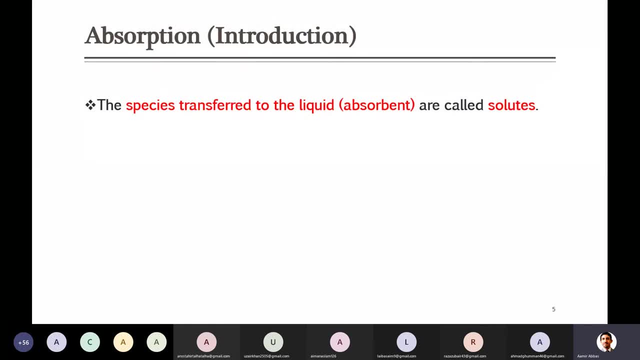 transferred to the liquid mean the all those components which you want to transfer to the liquid that you want to absorb inside the liquid. they are called cell. you before that mean this: the liquid are the solvent, it is called absorbent and later on we will be using actually these terminologies. mean: 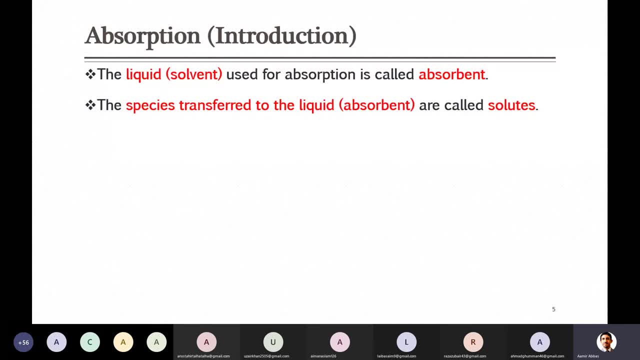 sometimes we do solvent liquid or if somewhere it is written absorbent, so absorbent is actually that liquid and the species that you want to get rid of or if you want to absorb. they are called cell you until unless they are not absorbed. but whenever they are absorbed, when salute has been absorbed, then they 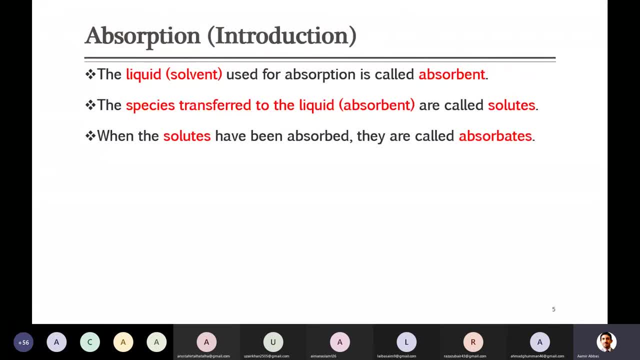 will be called as absorbents. okay, I think you are aware about these terminologies: absorbent, absorbate. can you tell me? if you didn't come across these, at least you have come across, I think, absorbent, absorbate. so in case of solid, because last time we discussed some wear absorption. 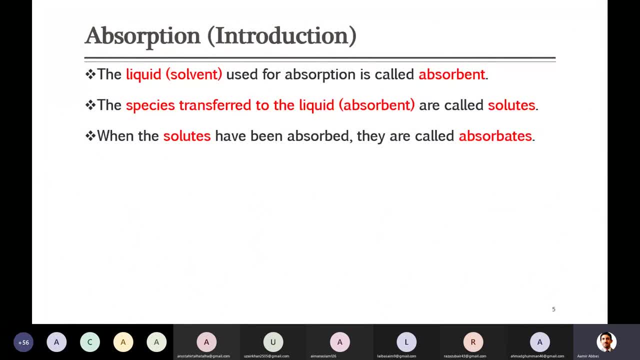 quickly, so solid material on which you are absorbing the thing that is called here, opposite to that, because liquid kept it, those species, those components, so it is absorbent and all those things which are absorbed are called absorbent. so then another thing which is called stripping, that is opposed to absorption. so what? 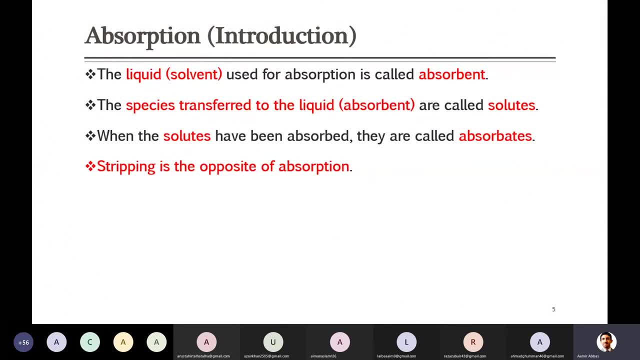 does this mean? so gas which we have absorbed inside the liquid we are removing the dead things which are absorbed into and then they can not absorb like we know it. there is a common assumption in approach to absorb my opinion to everything about object. so there's lots of arguments here and there. 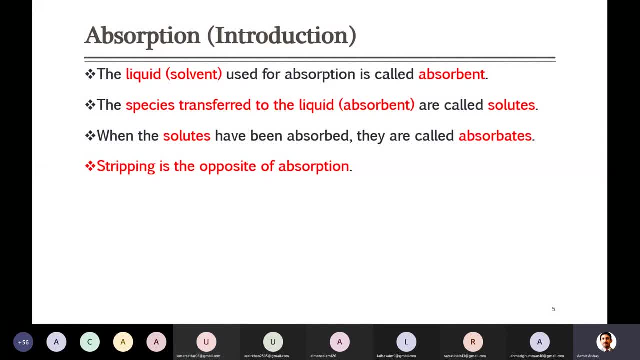 There has also my point that there are a lot of peopleitenrs, that some voluntarists have got way. sos sondern diephantisch diault. confirmation: good, Even by the use of Secza umaneous experiments have actually done that Good. So in absorption, what we were doing, we were capturing some of the component of the gas in liquid. So here, in the case of stripping, you will be just removing the components which are absorbed inside the liquid and with the help of some gas here, as Omar mentioned, 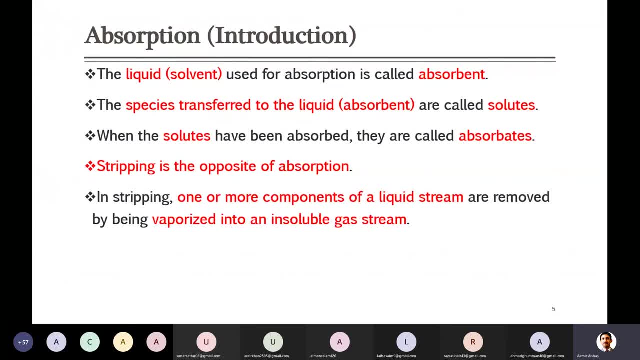 So in stripping one or more components of liquid stream, I mean, if you properly define it, it is the removal of one or more component of liquid stream. and how they are removed? They are removed by vaporizing into insoluble gas stream. 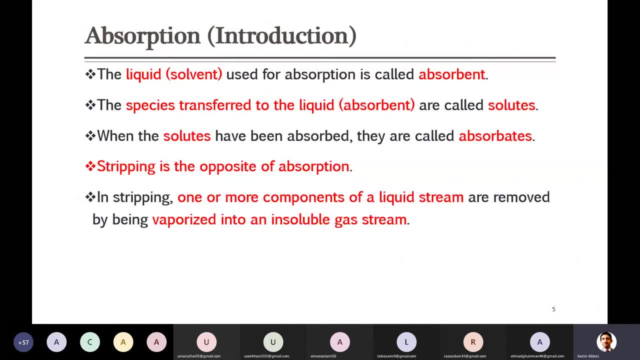 Insoluble here means the gas stream that you are bringing here as a like mass separating agent. Last time we discussed This that in absorption column as well as stripping column, there will be some mass separating agent. You have to introduce some mass separating agent stream, for example, in case of absorption, what is mass separating agent? 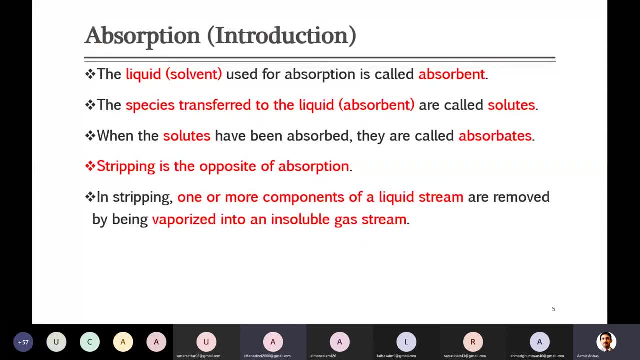 So the substance which is used to, Yes, liquid liquid which you are using definitely for absorbing the liquid stream introduced will will be called as a mass separating agent. And here In stripping then there is a some stream which is used to remove some of the component and that that is here the gas. 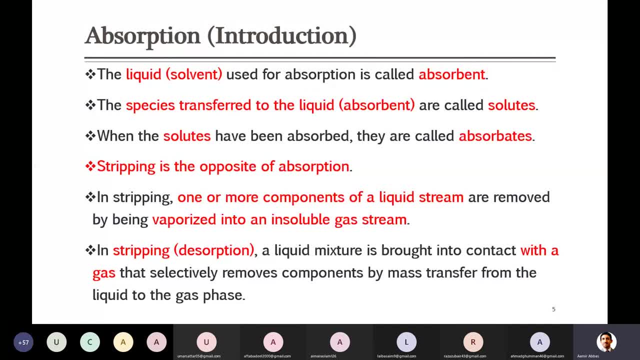 So that will be mass separating agent. So in this case of stripping, or sometimes you can also call it, or you, you can come across this- I mean this name, that these options, they also call it these options, absorption and these options. So this is not widely used, but some in some text, you can come across this. 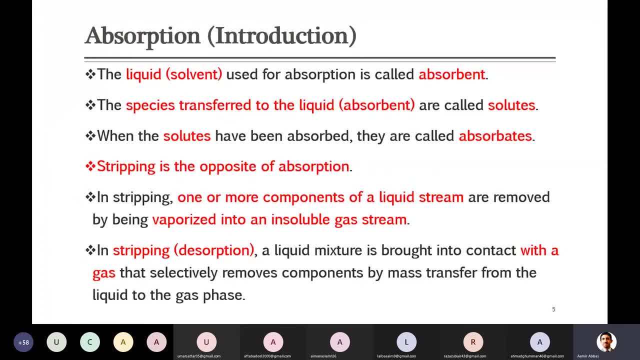 So I mentioned here. So in case of this stripping or desorption liquid mixture you bring it contact with the gas and that gas selectively remove some of the component by mean from that liquid phase, not all the components. and here the purpose will be actually to remove mean to recover or regenerate the liquid so that it can be used again. 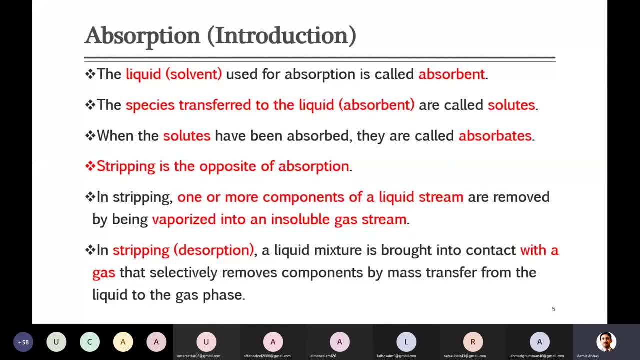 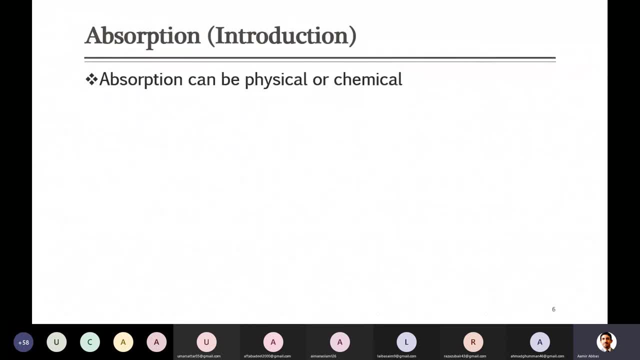 I mean in the absorption column. So absorption can be of both type, physical as well as chemical in case of physical absorption. So what does this physical absorption mean? The nature of is: when you absorb on the don't chemical protection takes place Right now. 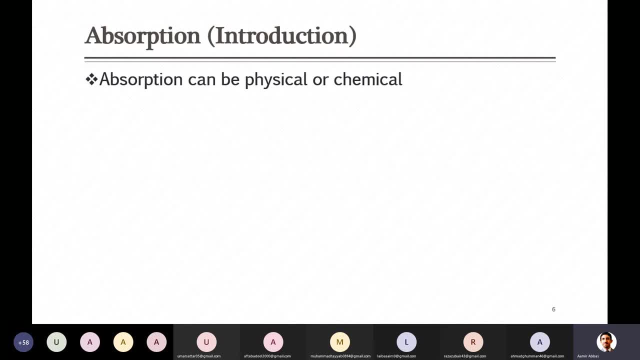 Chemical reaction takes place and they get absorbed the help of weak bonding forces. and those weak bonding forces can be like hydrogen bonding. there can be something you can say dipole moment, and some kind of weak forces which you studied somewhere are there in fsc or maybe in chemistry courses, so they act here in physical absorption. 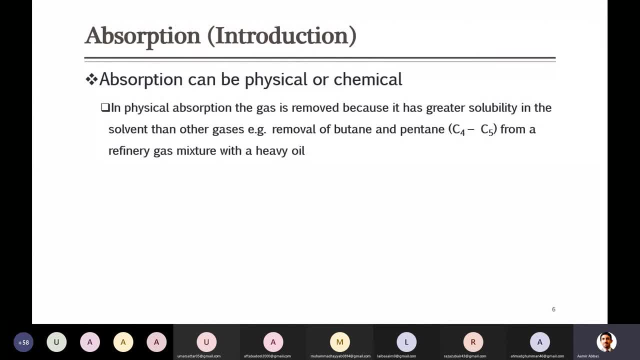 so in physical absorption gas i mean absorption which means we are removing some components of the gas. so here the gas is removed. all those gas components which have a good affinity towards the liquid they are removed, and here the forces are simply like weak bonding forces. there is not. 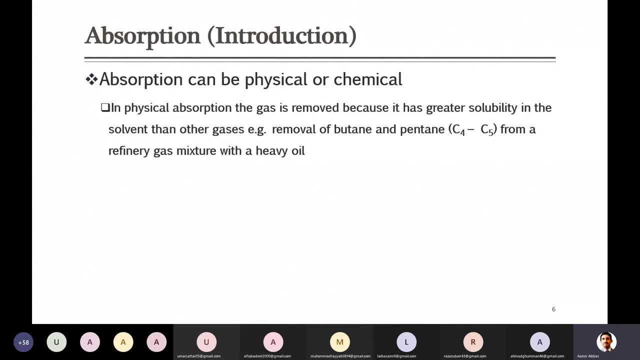 proper bond formation due to weak bonding forces like hydrogen, uh, hydrogen bonding, uh wonderwall forces like these dipole moments and such kind of forces. they help you uh, i mean, and actually when something has as affinity towards the liquid actually that develop these weak forces with that liquid. 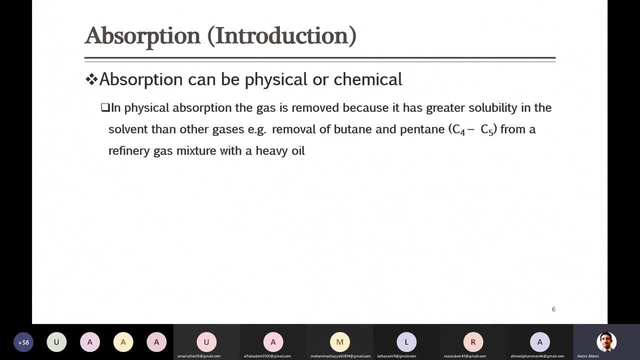 and gets removed from the main gas stream. for example, here mentioned is butane and pentane, so they are somehow lighter hydrocarbon and they are removed from the refinery gas mixture with the help of heavy oil. refinery gas mixture consists of, for example, gases starting from c1 to c5. 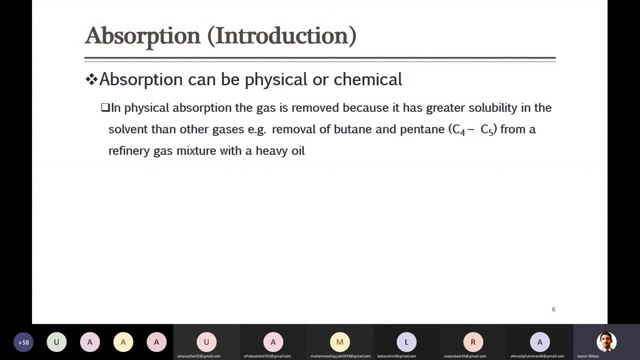 c1, methane and so on, with hydrogen and such kind of gases. so if you have to remove these are a bit heavier components. butane and propane, uh, so repentin. so they are removed with the help of heavy oil, and the heavy oil is, i mean, i'll, it's, it is, uh, i didn't know what does this heavy i mean? 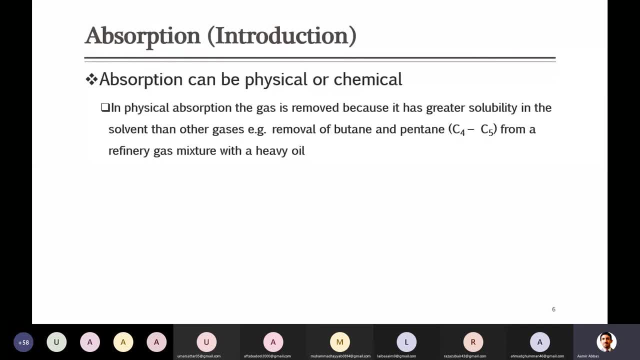 light and heavy and somewhere i think you are studying energy engineering this time. so actually i uh, uh, uh, i okay. so so enough again. so okay, go, go and hit, okay, gases in refinery. so in other way, the opposite, one opposite to this physical, is the chemical absorption. so in case of chemical absorption, there will be a 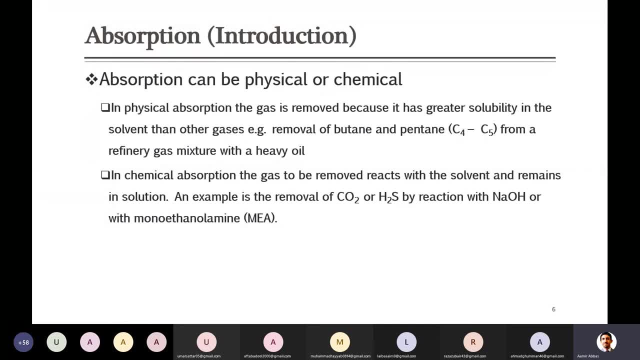 reaction between liquid, because it is absorbed as well as the absorbent which you want to absorb here, the gases. so an example here is the reaction or removal of co2 and actually h2s, either from natural gas or maybe from biogas and so on. so there are, removal takes place with the help of some reaction. so these two 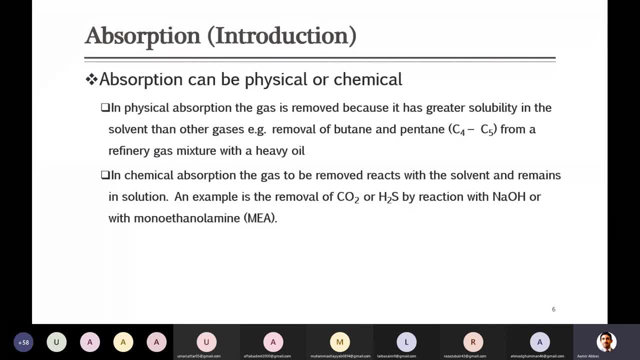 Co2 and h2s. they can be removed with the help of both adsorbent mentioned here, like NaOH and monoethanol amine. so in both cases here either you are using NaOH, so noh can be used for removal of both of these species as well, as mea can be used, but preferably 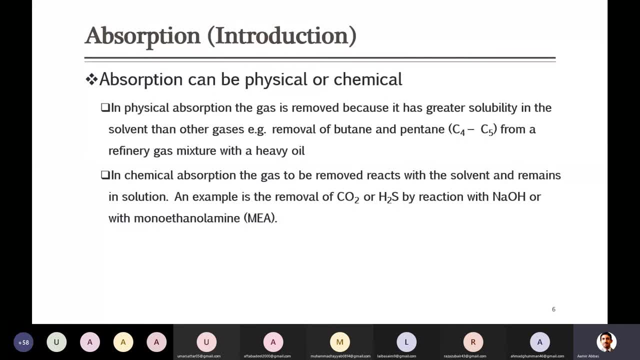 noh is more, more good or can remove h2s in a better way as compared to- i mean like this mea, and mea is good for removal of co2, as already i mentioned. so in this case there will be a proper bond formation. so that is called chemical absorption, and when there is a mean chemical 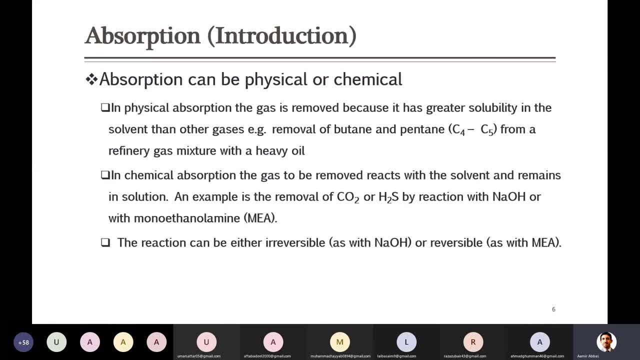 reaction. so there are two types. you already know that there can be reversible reaction as well as irreversible reaction. so in case of here, anyway, when it reacts with either co2 or h2s, and usually this make a mean permanent bond that is irreversible as compared to this. 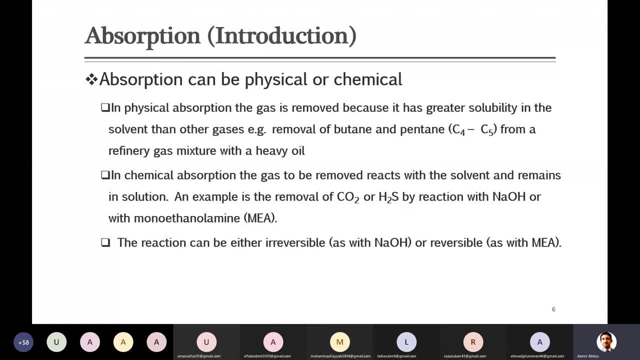 mea that makes a bond which is reversible. we can reverse this process for irreversible reactions, uh mean, uh, that is preferred one. sorry, reversible is prefered one. the reason is that we can regenerate the liquid, we can bring it back to the absorption column, while in case of irreversibles- irreversible and you cannot regenerate, neh when it has reaction. 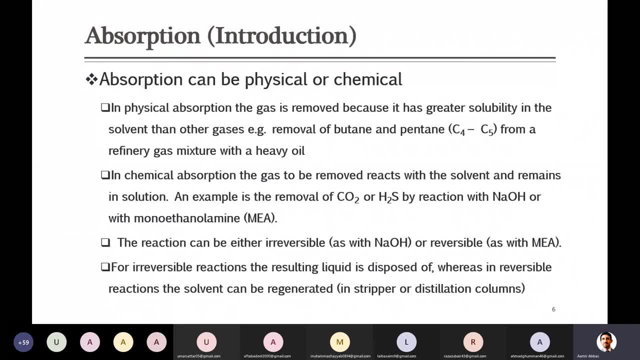 when any of these, either H2S or CO2.. So that makes a chemical that you cannot reverse the reaction. If you want to even reverse it, that will be either too costly or that will also not regenerate the liquid. It will be broken down into something else. So in those 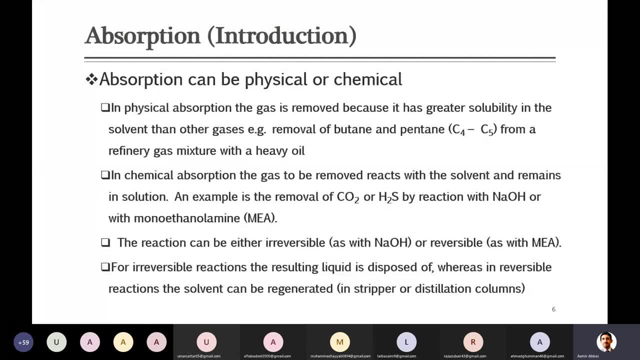 cases when it is irreversible. always you will need new liquid, But in case of reversible reactions we usually regenerate the liquid. and how we can regenerate that is in the main like stripper or distillation column, And in that case maybe not only with the help. 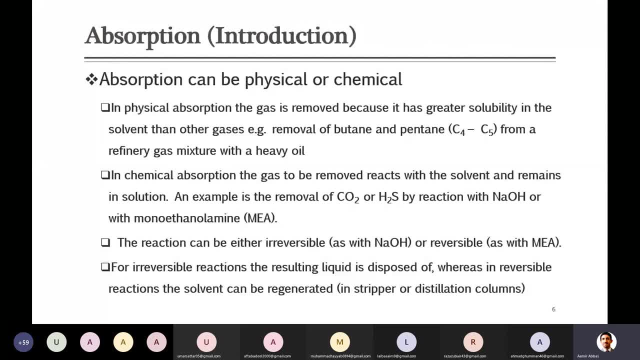 of only passing some gas. sometimes you will need extra assistant in terms of heating or like this, So you can regenerate those liquids. And what will you prefer, by the way, in such case? either it should be reversible or irreversible. But before that, physical or chemical, Which one should be better, in your opinion? 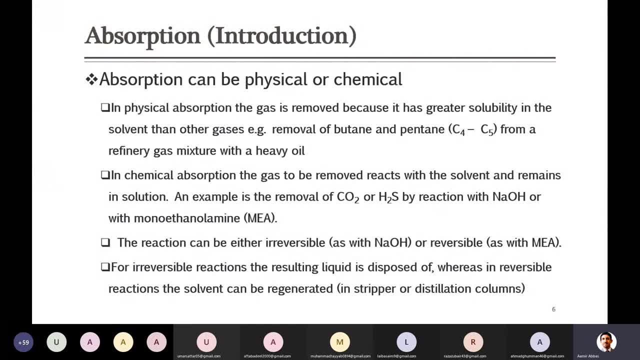 Physical, I think. Physical sir. No, any other answer. I mean, actually, I'm asking in this way that which one will give you more absorption, physical or chemical? First of all this one: Chemical sir, Chemical sir. 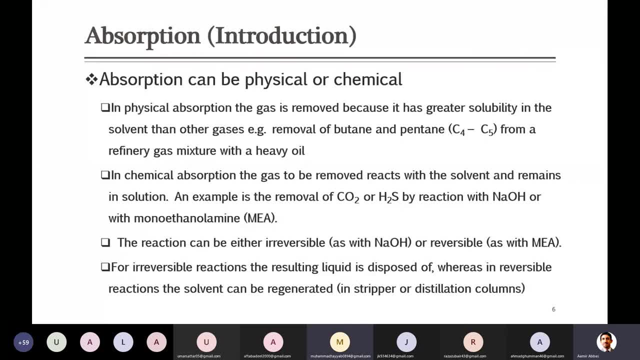 Chemical, sir. Chemical In case of chemical because, as I mentioned already, in case of physical guys there are very weak forces. So that will not generate good absorption until unless some bond formation is taking place, And that will be a bit good absorption, Yes, when there. 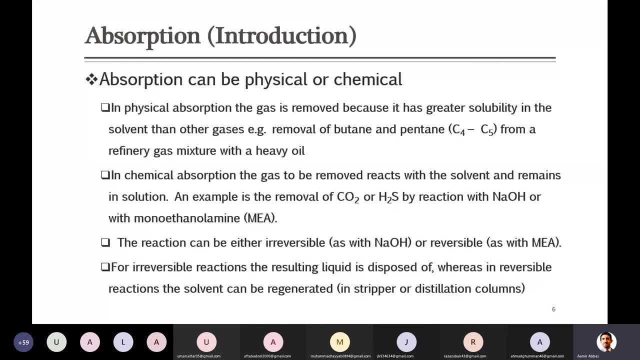 is a bond formation in case of chemical absorption. later we will discuss it somewhere in detail, hopefully. So in case of chemical absorption the absorption will be very good And then the absorption will be higher as compared to physical. So due to this reason we will 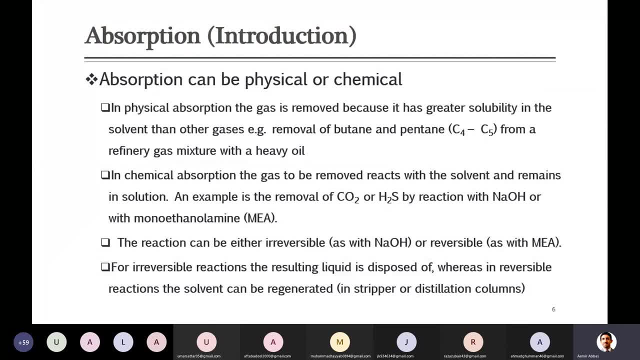 prefer it chemical. But in chemical, as we mentioned that, there are two categories. Now, out of those two categories, which one is better? Which one you will prefer, Sir? separation wise, irreversible will be better, But cost wise, we will prefer reversible. 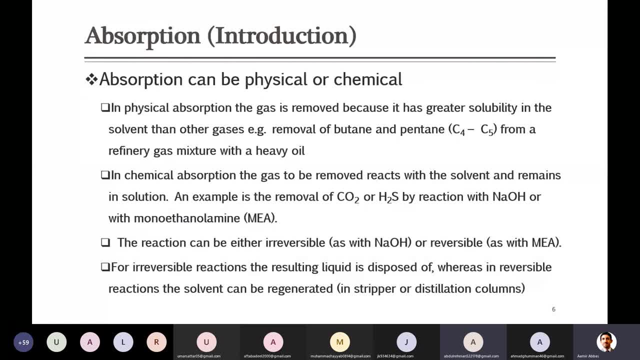 more? Yes, but you are right. But the reason is irreversible, Yes, Irreversible. if you are getting something when you are absorbing some of the gas and you are getting some species which is of good value, like that has some, I mean that can. 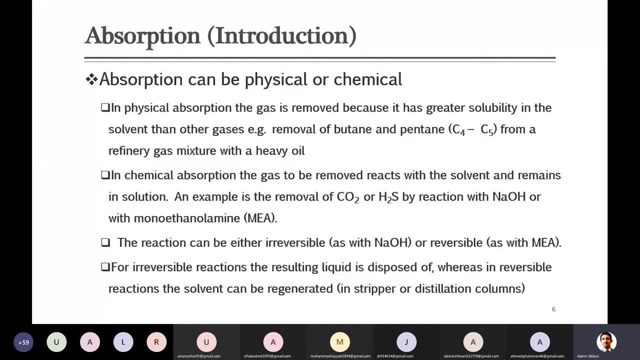 be sold at good cost, So at the higher cost as compared to your solvent. In that case, it is definitely good to go for irreversible, because you will not need another equipment to get it separated and bring it back And at the same time it is giving you something. 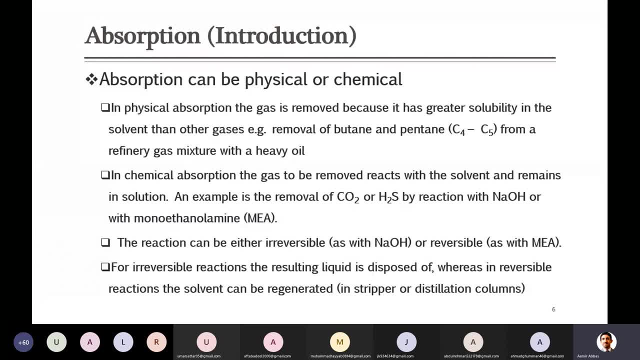 valuable, But I mean most of the cases. the products which are obtained are not that valuable as compared to the liquid which you are using for absorption. So we prefer reversible cases so that we can regenerate and reuse them, because liquid- for example these monoethanol amines- 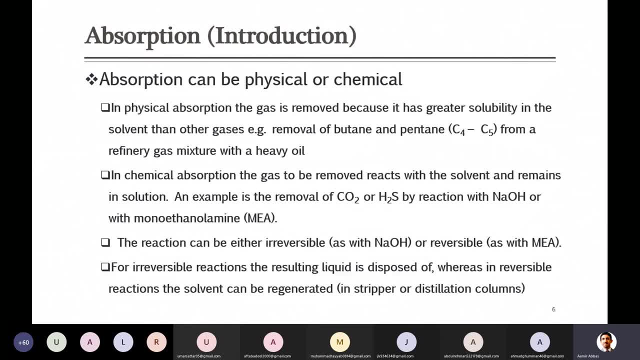 anyway, definitely they have cost. They are not like cheaper, They are not like water, simply that you are using it for the absorption. So due to this reason, most of the time in the industry- I mean- reversible is preferred so that that can be regenerated and can be reused. 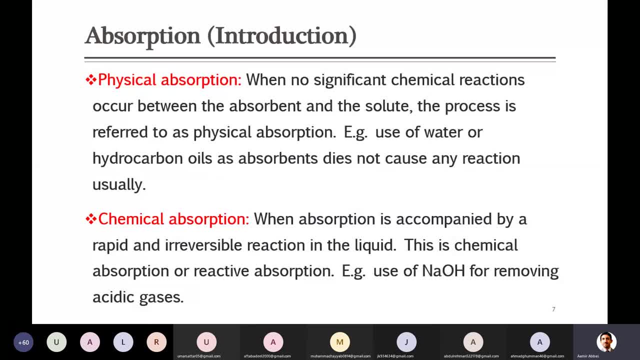 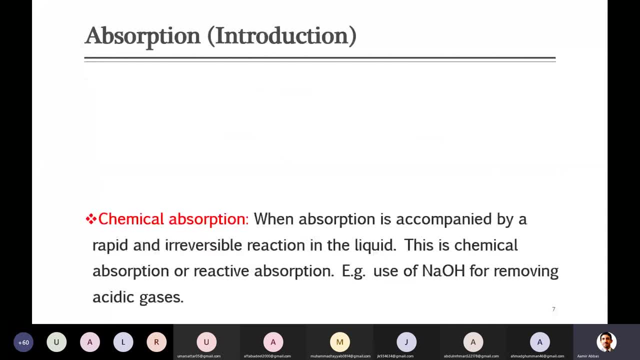 So more or less same thing is again mentioned here in physical, like absorption I already mentioned, because in the last slide here I have directly written that what is happening. But what are the examples? in this case I think the same will be mentioned, but no significant. 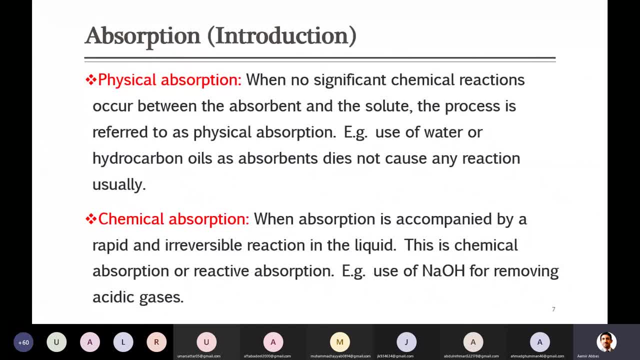 reaction takes place and weak bonding forces. in case of physical absorption And in this case, for example- here it is mentioned use of water or hydrocarbon as absorbance, They come in contact and they are used for the absorption. So that's physical mainly, And 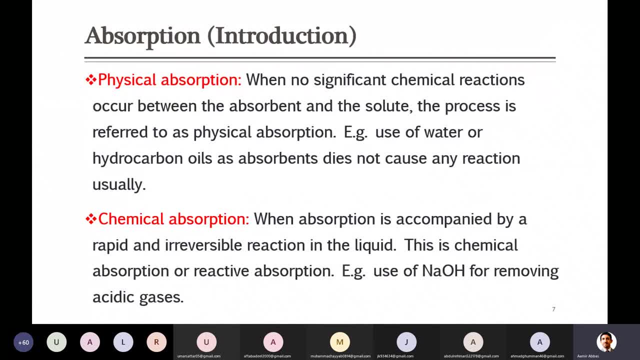 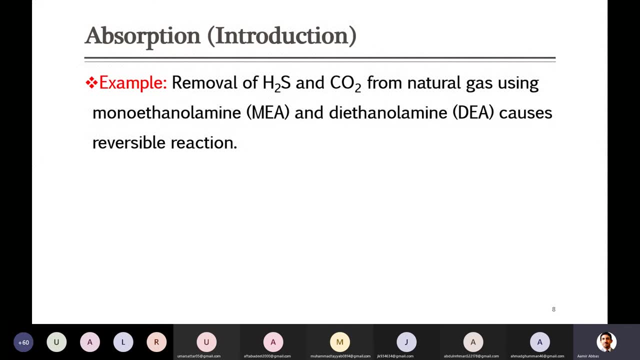 in case of chemical absorption, when absorption is accompanied by rapid and irreversible reaction mentioned here, irreversible like are maybe reversible reaction. both can be used. So the same example of NIH. So removal of H2S and CO2 from natural gas, using these by the 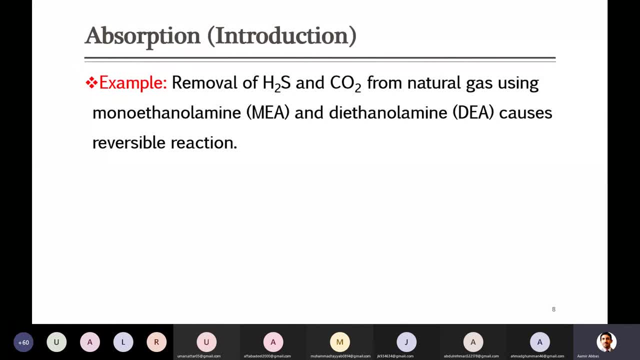 way already mentioned this monoethanolamine, diethanolamine, even triethanolamine, So they are called, usually a mine solution and they are very widely used in the industry, this natural gas industry, for removal of these contaminants. Now, chemical reaction actually increase the rate of absorption and solvent absorption. 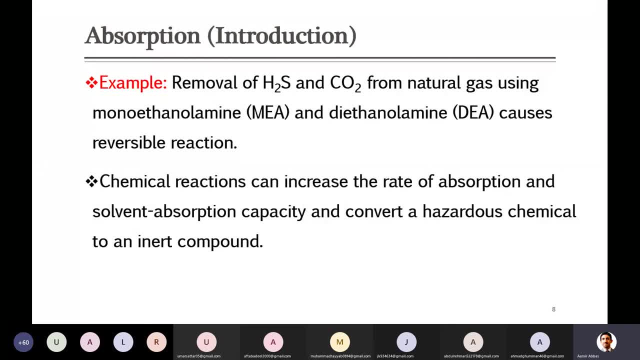 capacity and that convert a hazardous chemical sometimes to inert compound or the compound is less hazardous. So through this this is preferred chemical one because first of all, rate of absorption is higher. And when rate of absorption is higher, definitely by using some small amount of even absorbent you can get mean more absorption as compared to. 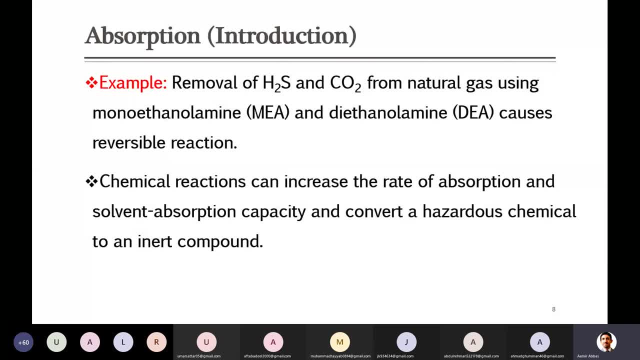 the physical, For example, we are bringing the same amount of two liquid- One can go for the physical and other for the chemical. So in case of chemical absorption will be higher with that even same amount. So at the same time as he mentioned one other advantage, 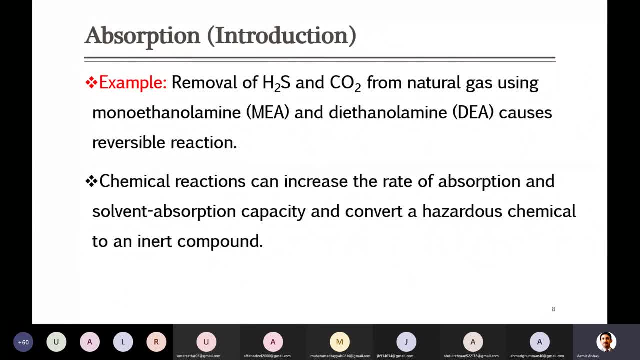 of this chemical is that, due to chemical reaction, sometimes hazardous pollutants are converted to something less hazardous, For example in case of H2S when it is reacting with the NaOH. so it produce, sometimes sodium sulfide. I think they call it, Yes, sodium sulfide. 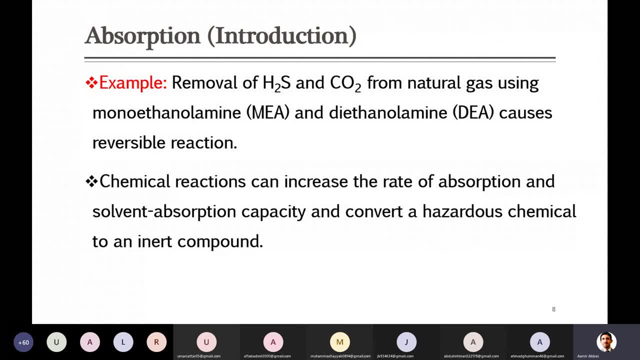 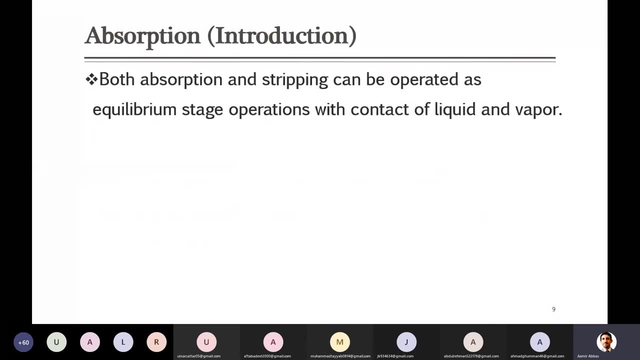 and sodium bisulfide. Actually it will be something Na2S or NaHS bisulfide or sodium sulfide, So that's less hazardous as compared to the H2S. So that's, that's what he means. These absorption and stripping- both are actually operated as equilibrium stage operation. 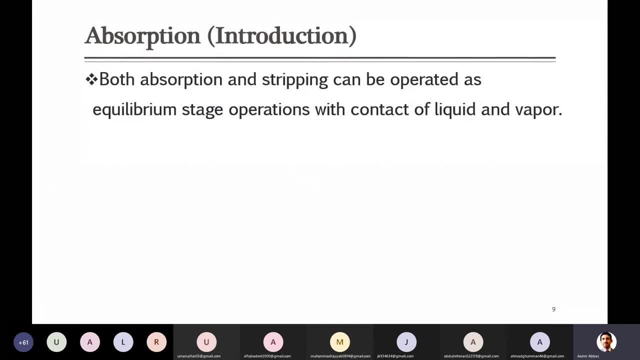 in which we bring in contact, as we discussed, that there is a liquid and vapor. They are coming in contact, as we discussed. I mean, what is absorption, What is stripping? In both cases, you know that there are always liquid in the gases, liquid in the vapor. 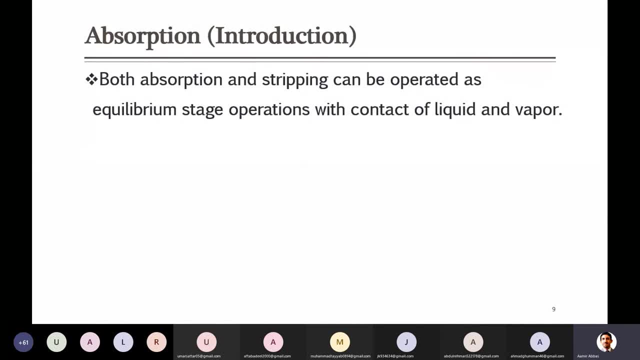 They are coming in contact. So there should be some equilibrium stage operation in which liquid and vapor come in contact and they lead to some equilibrium and then move to the next stages. So, as you already studied, I mean whenever there are like these vapor. 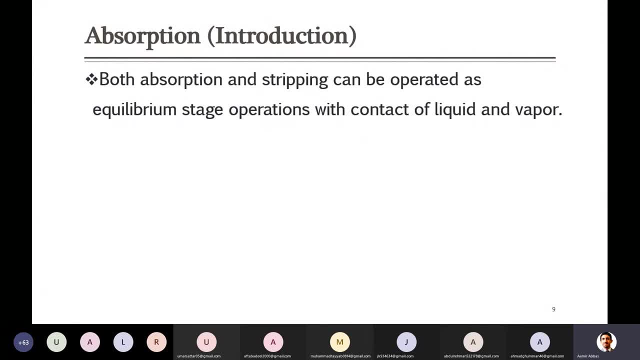 liquid contact and equilibrium stage operation, then in case of that is somehow case similar to the distillation, because in case of distillation also we bring in contact the liquid and vapor and we go for equilibrium stage operation And as you used in distillation, there can. 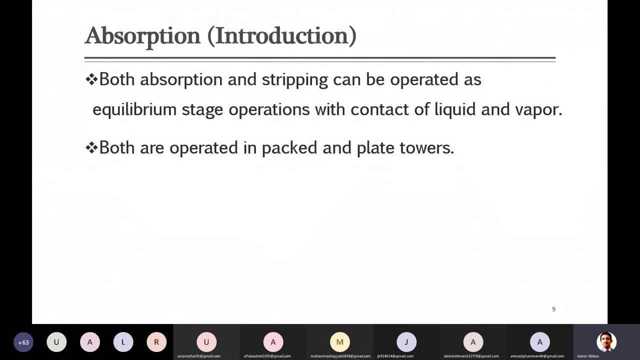 be the, or you studied that that can be carried out in form of packed as well as plate tower, Although in case of distillation commonly plate towers are used, but both can be used. So here, in case of absorption and stripping, the same. I mean equipment which are packed. 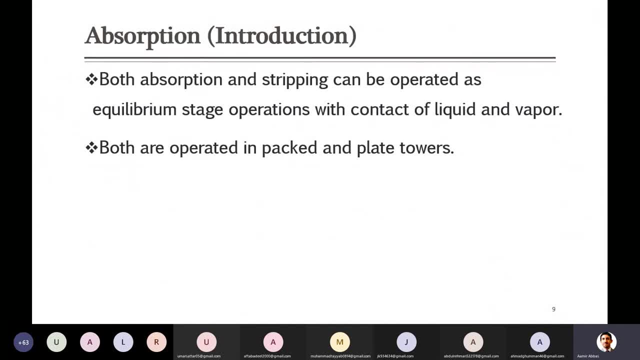 tower or plate tower. they can be used to bring in contact the liquid and the vapor. So when you are bringing in contact these main liquid and vapor in absorption and stripping, so here the small difference from actually, I should say, with respect to distillation. 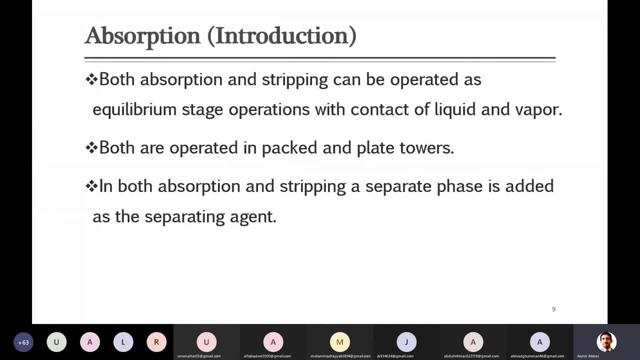 their difference is here in absorption and stripping, although we will be using packed tower as well as plate tower, but in case of absorption and stripping always we introduce a separate mass separation Again, which is not usually introduced in case of distillation. 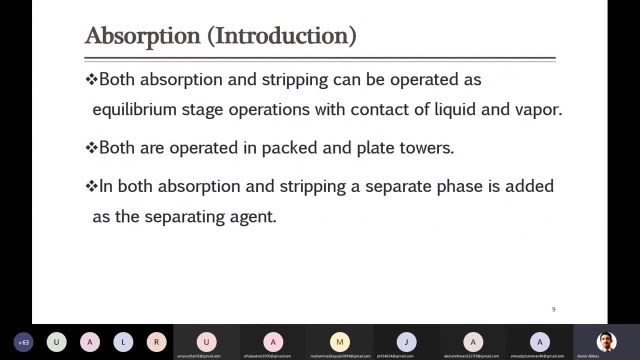 So that's a one difference from that that you have to introduce some mass separating agent in case of this absorption and stripping. So when we are using this stripping agent, so their column which is used for absorption and stripping, that column is simpler as compared to the distillation. 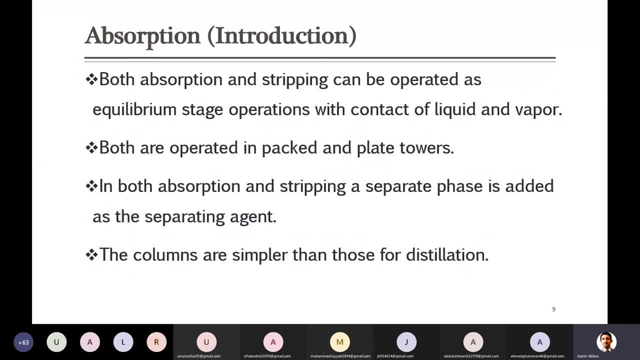 Actually, in case of distillation column, we have to use condenser as well as reboiler for reaching to the separation or to make or to achieve that specific separation. But here, in this case, when you are using absorption and stripping most of the time, 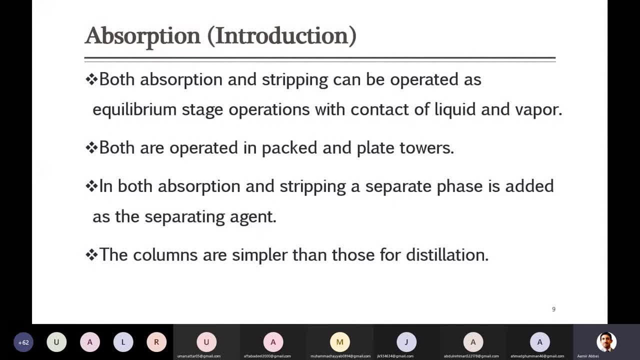 there will be some straight, simple column in which you are introducing your mass separating agent and bringing other species in contact with that. But in some of the cases, based on your process, you have to use condenser. So this is based on your process requirement. 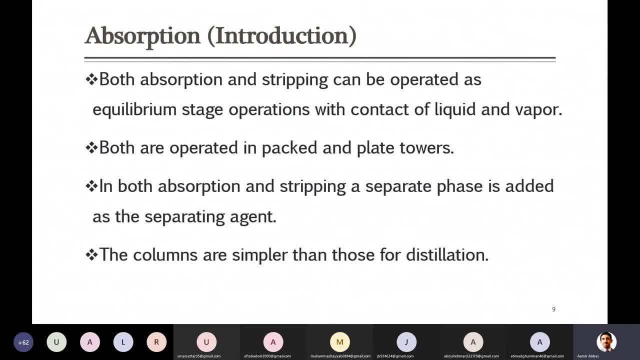 Sometime you can use like condenser at the top of this column. One student has asked this question in the chat and that was related to this, I think, stripping reflex column. So that was simple stripping column, But at the top of that there was a condenser. 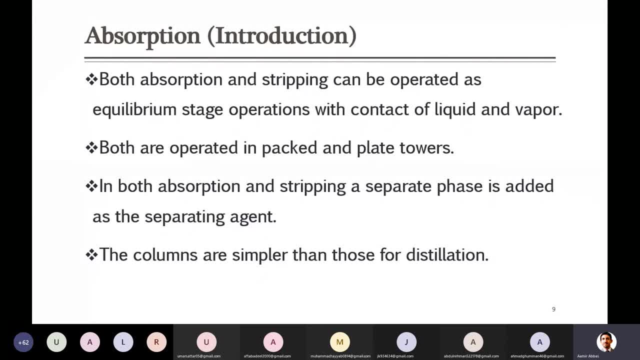 So some of the liquid was being, I mean condensed vapor, which were reaching to the column. They were being condensed And that was reflex, Reflex back to the column. So at the same time in some of the conditions- maybe you will look at the bottom of the regeneration- 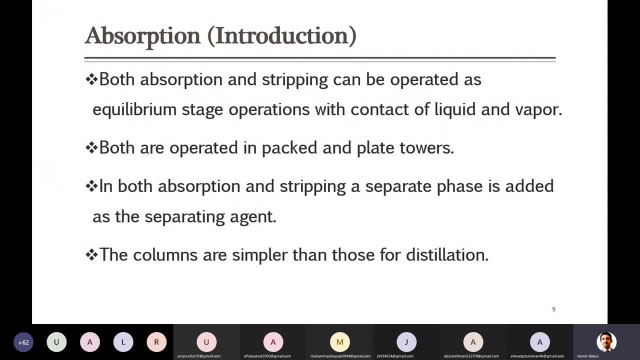 which is stripping section at the bottom of that. Sometime you can have a reboiler. Actually, the purpose there will be to provide some of the heat for disengaging or removal of the components from the liquid which we want to get rid of. 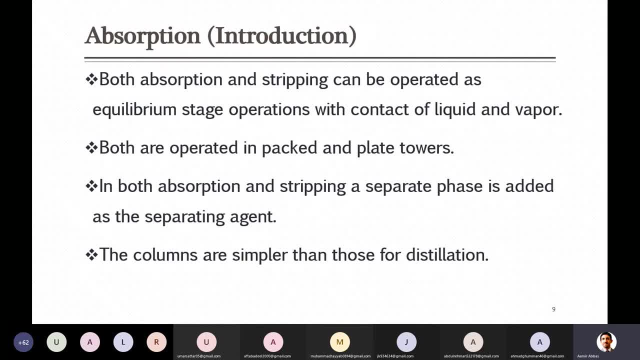 So that liquid can be regenerated. So, but most of the time they are simple column. They don't have these mean like regenerator as well as condenser, So due to this, they are as simple as compared to the distillation unit. 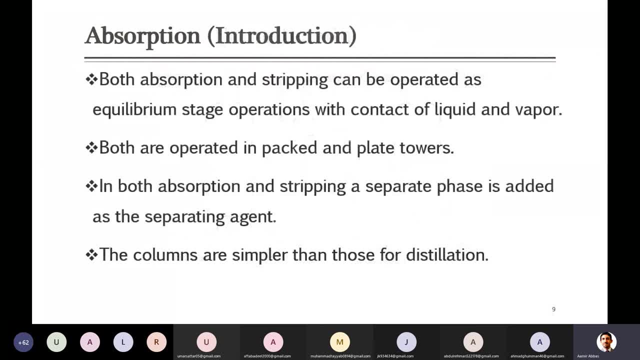 As up to here we have talked about the absorption. So in case of absorption, when I go after defining the absorption stripping, then we come towards the type of the reduction And they were physical and chemical And, as I asked you, that out of those chemical is better because with the same amount of 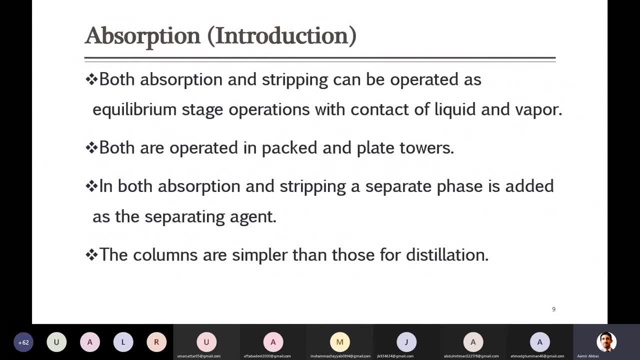 liquid you can get more absorption as compared to the physical case. So in case of chemical, as we discussed, that out of reversible and irreversible, the preferred one, the most, which is commonly used, that is reversible. In that case reversible means we can regenerate the liquid. 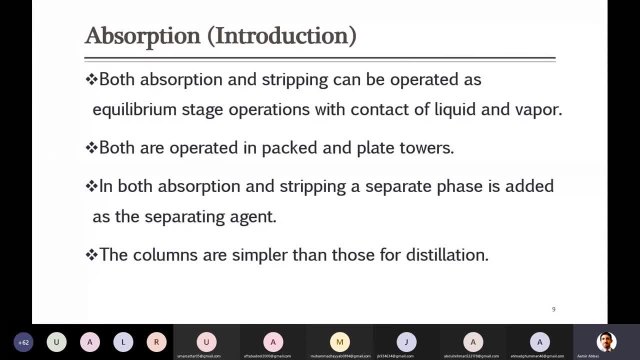 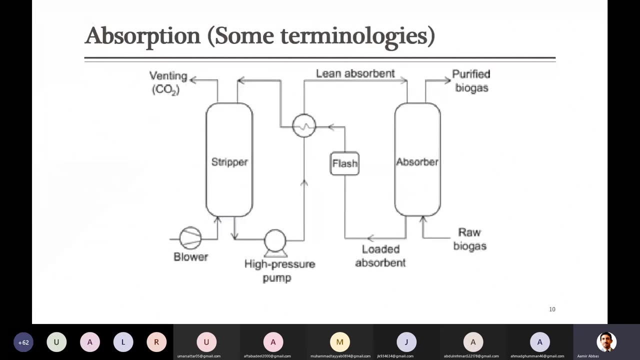 We can just get rid of those species which were absorbed inside the liquid and then can bring it back to the absorption column again to recycle it or to reuse it. So here there is one example in which they are shown together like absorption and stripper, because these both operations goes in parallel, like in case of absorption, if you look at 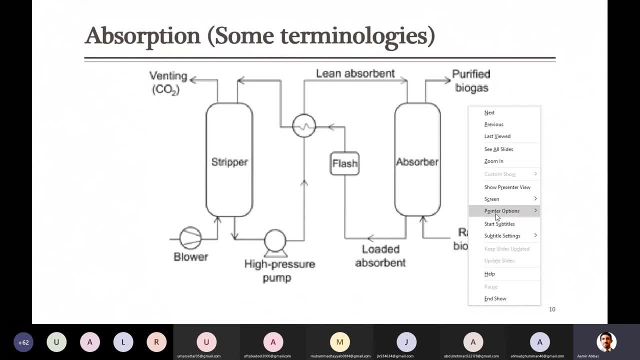 this diagram. Actually, it is somehow reverse: Absorber should be on the other side. Yeah, So maybe we will keep getting confused. But okay, just look at this. This is absorber, in which what you are bringing is raw biogas. 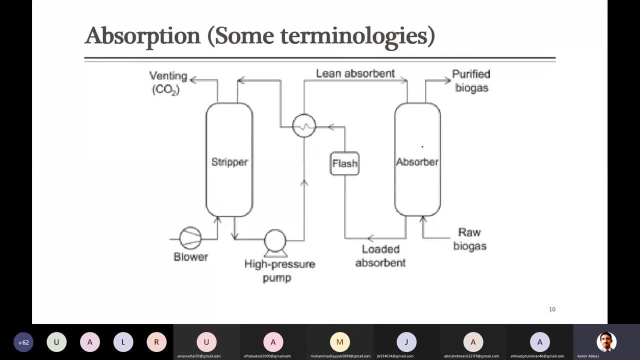 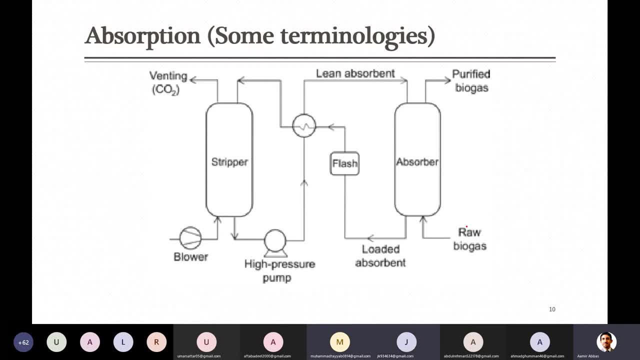 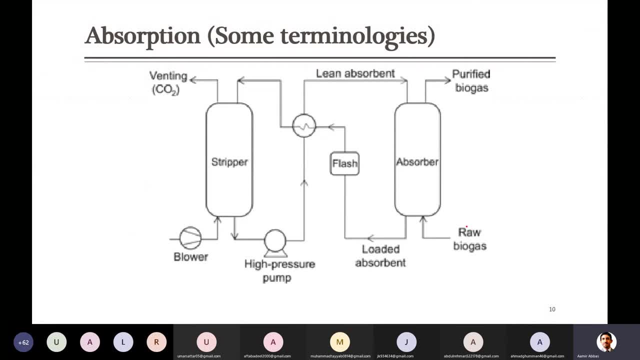 So I guess because this produced by a from that biomass in the absence of oxygen is called biogas and that that contains Actually. maybe we could use that later. Yeah, We could. you have come across some of the news that biogas plants are installed in the village so that 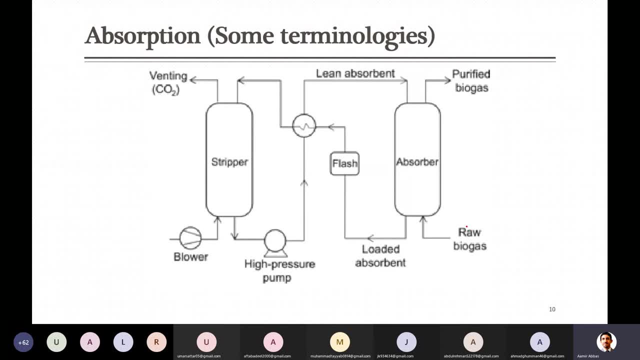 they can just use animal waste and can produce this gas. and that gas can be used, uh, for cooking purpose, i mean for burning and cooking like, so i mean biogas. actually, its composition is mainly like the ch4 natural gas. uh, then can be co2, h2s as an impurity. they 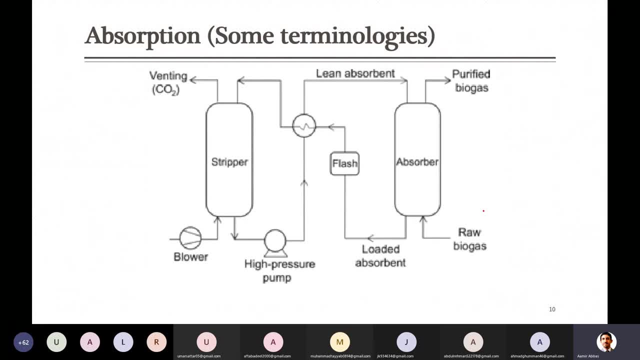 are present in this. so in this specific example actually we are just talking about presence of co2 in the biogas, but generally speaking, uh, there is self are also present there, so h2s is also part of this, but here the purpose is to remove co2 in this example. so in this example here, draw biogas. 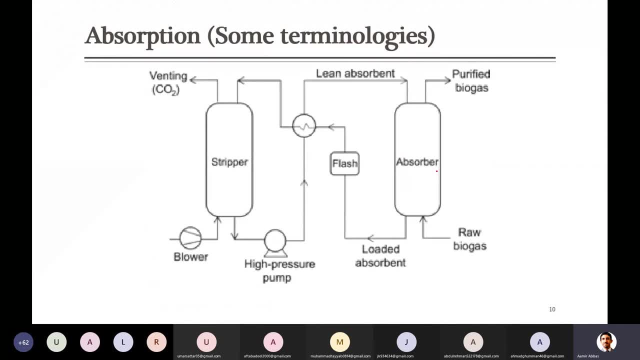 enter to the absorption column, so in this absorber or absorption column, in order to remove some of the components, and i, as i mentioned that here, the purpose is to remove co2 from this gas. so we will bring some liquid in contact with this. this from the top, you can see. i will just 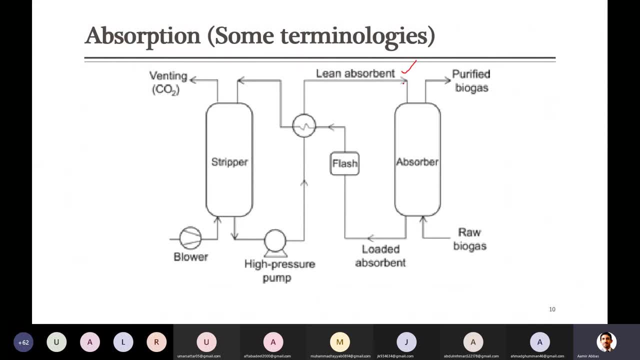 tell you what is this? lean something. so i just simply just consider that in this column, the gas is entering from the bottom and the liquid will be entering from the top. so, uh, the gas being lighter, will move to the top- i mean because it is entering at the high pressure- and the liquid will come down. 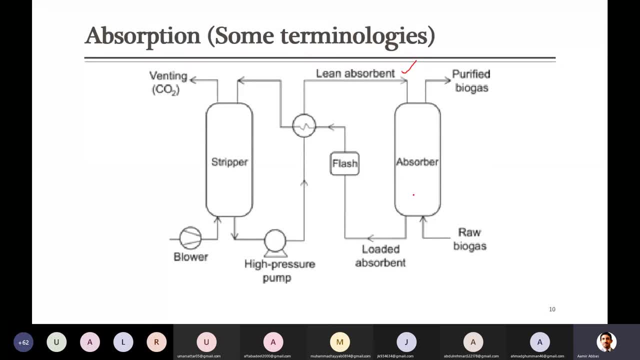 to the gravity when they will come in contact with each other. the purpose here is to bring such a absorbent that that can absorb co2 from this gas. so when we bring it in contact with that liquid, that is, i mean, that has affinity towards co2, that that will absorb co2, and that is mainly like mea. 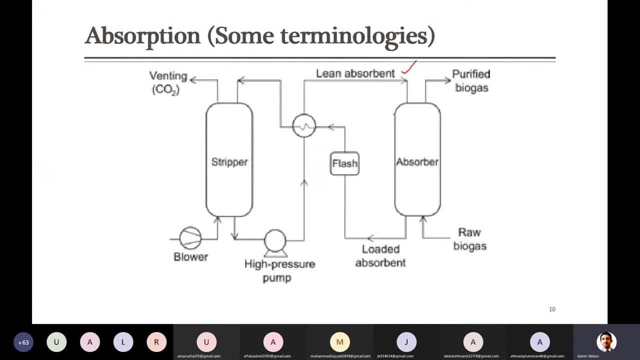 that is very commonly used to remove co2. so let's consider this mea. that will absorb uh co2 from this and at the end it leaves from the bottom, while the gas which is purified- which purified means those impurities which you were supposed to remove. they has been removed in this column so that liquid comes to the bottom. now that liquid we 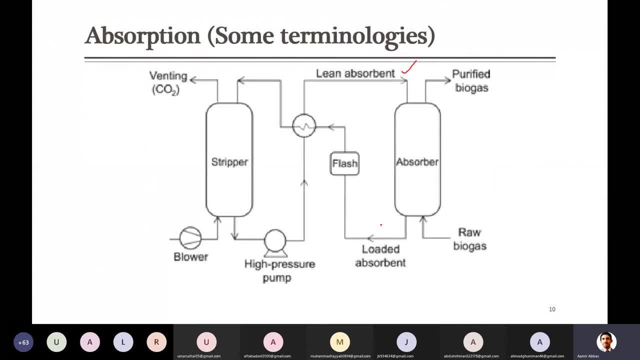 said that is better to regenerate the liquid, to recycle the liquid so that it can be regenerated, in order to regenerate it where we will, uh, take it? we will take it to the stripper column, uh, i will just let you know. what are these things in between? so, uh, just before that, look, here it comes to the 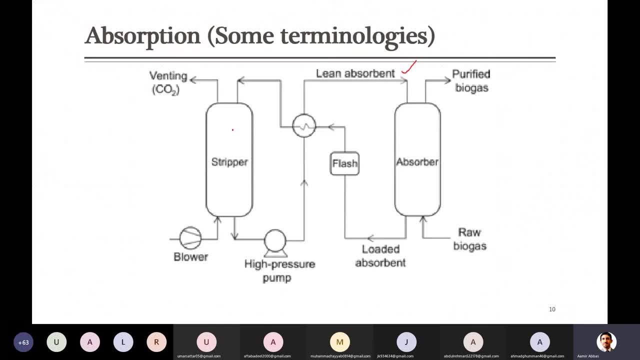 stripper and the purpose of stripper was to remove some of the component of from the liquid stream with the help of some gas. so this liquid will be, i mean, just thrown from the top. it will start moving down and you just introduce some gas. maybe sometimes you are introducing some steam, so steam, 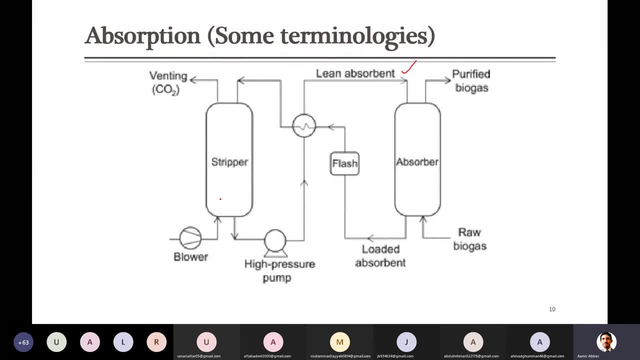 at high temperature and pressure so that it can reverse that reaction. it can. just, these are those components which were absorbed inside the liquid and they will be stripped out to the top, while the clean liquid will leave from the bottom. so then i mean here- this is the main operation- what is happening in case of absorber as well as in in the stripper? here, 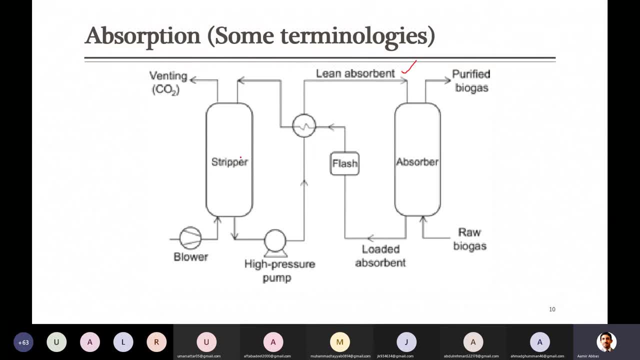 the gas come in contact with the liquid and gas tips out. uh, those components which were just carried out so that they will not be act as a stripping agent and the next thing we will do is to remove the liquid that will strip them away. so here, as mentioned, is venting co2, so you will be 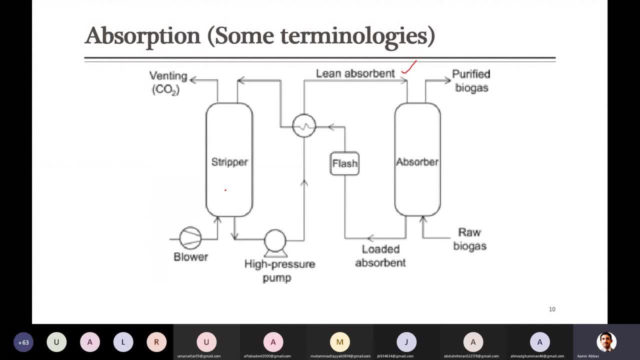 just bending co2 with the help of some gas. that can be like you can just introduce air from the bottom or most of the time steam is introduced inside the stripper column. so because steam uh will be like providing heat as well as that will be acting as a stripping agent. so 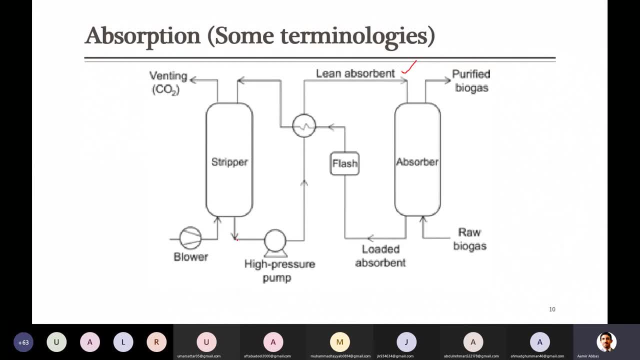 the clean liquid. so actually, this clean liquid that should be sent back to the absorber. and this is how it works continuously: that, like liquid which is initially started from here, you will bring some storage and it will be pumped and you will bring it to the absorber. so why a pump is being used here? can anyone 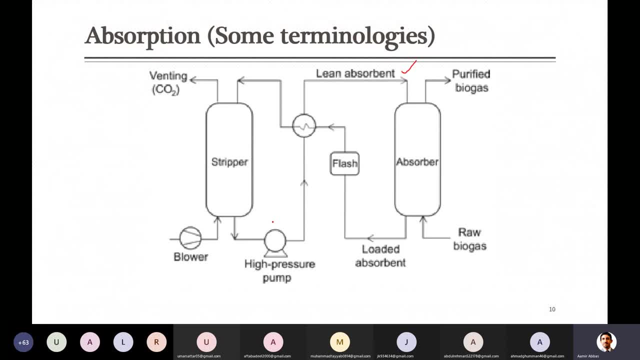 tell me the reason to use pump. yes, good, first of all, the liquid solid point height. definitely absorber will be a column and this will be a long column. so in order to reach this liquid to the height, definitely you have to use some pump. but at the same time, in case of absorption, we discussed somewhere. 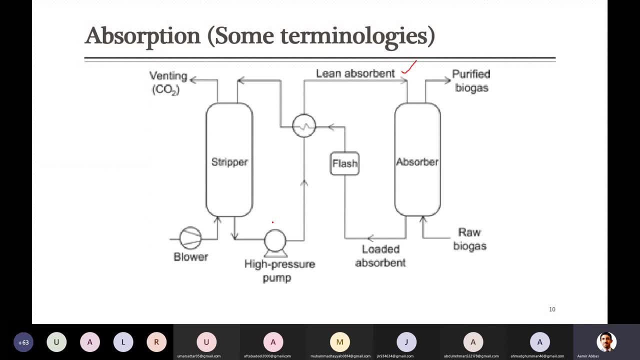 earlier. either we need high pressure or low pressure for absorption. which is favored, which is better for us. that is high pressure, high pressure and ambient temperature. yes, high pressure and exactly ambient at low, low temperature. so in this case, pump will also be needed to bring it to the light- high pressure. so the reason is to 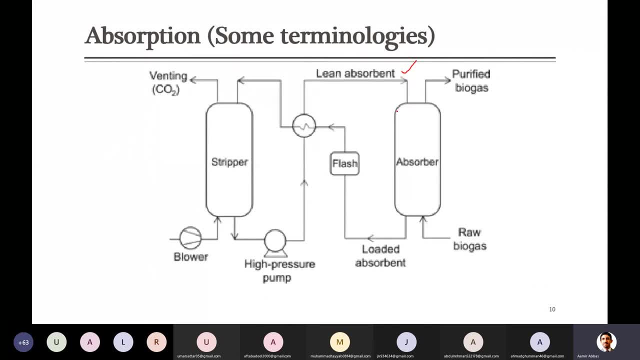 install pump here so that you can just send it to the height as well as to the light. it should be at high pressure. So here this is a heat exchanger. The purpose of this heat exchanger is to reduce the temperature of this stream which is going to the absorber, because we need low temperature in the absorber, while in case of stripper, we need high temperature, so that something is already stripped out, removed from the, because it is high temperature that favor stripping and that is 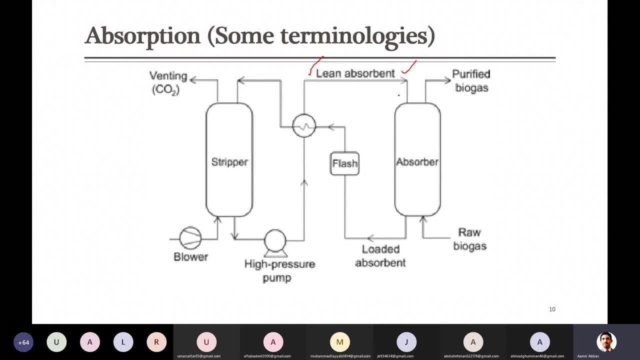 opposite for absorber. So for absorber temperature should be low. so we reduce actually the temperature of this stream which is going to the absorber, while the other stream, which is going to the stripper, we increase its temperature. So their heat exchange usually takes place. with that, here somehow some degree change in the temperature of both stream will be taking place, and then it is entering to the stripper, While the stream of the liquid which 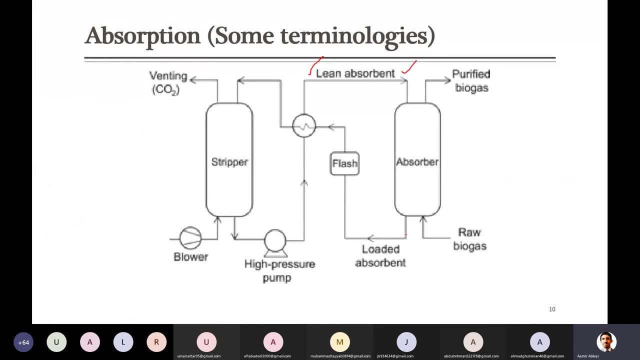 enters to the absorber. after absorbing species it leaves from the bottom, it is still at high pressure. So in case of stripper, stripper is opposite to absorber and in this case the pressure should be low. So what you do? you just install a like simple valve or you flash it so that the pressure of this stream, which was coming at the high pressure, that can be reduced. that can be. I mean, you can. 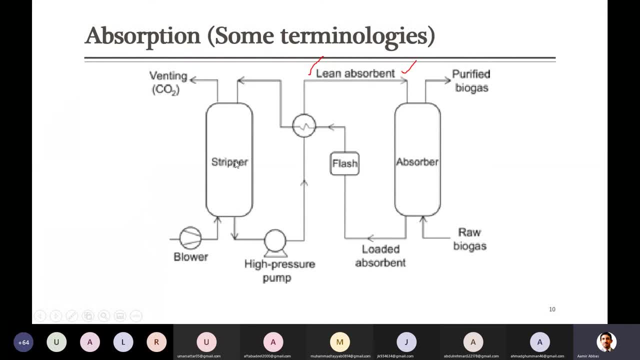 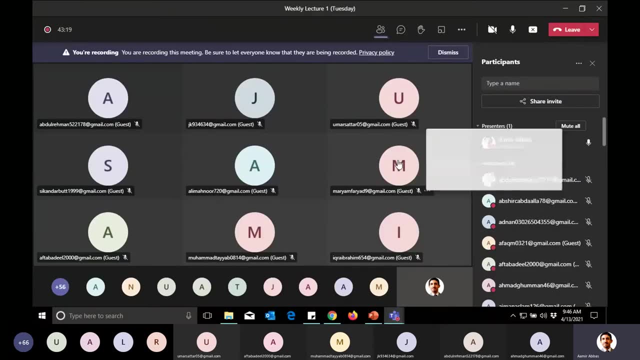 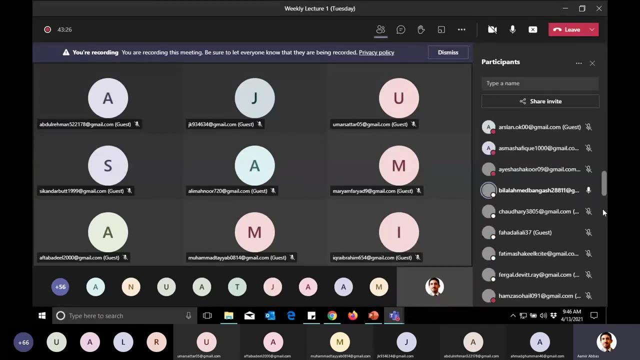 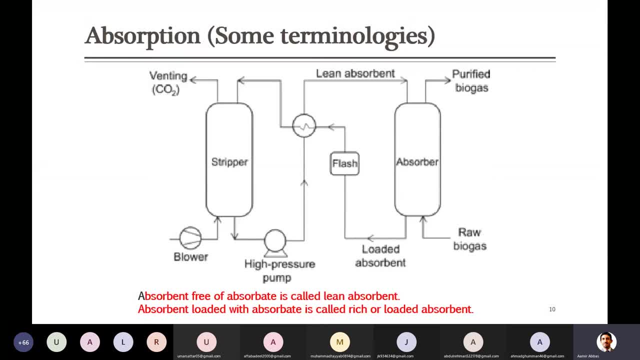 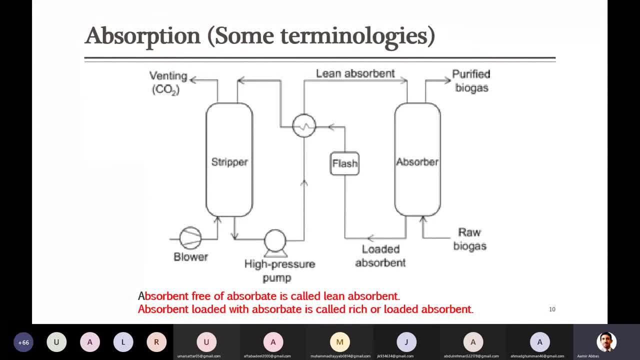 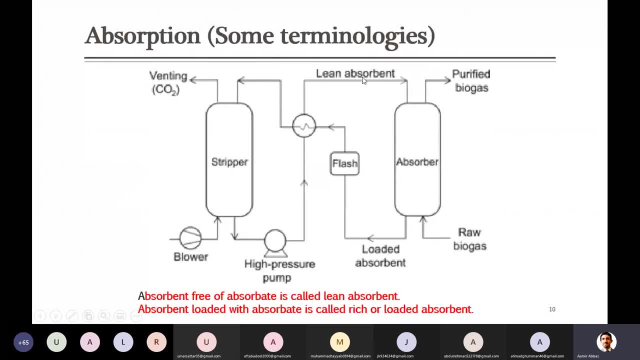 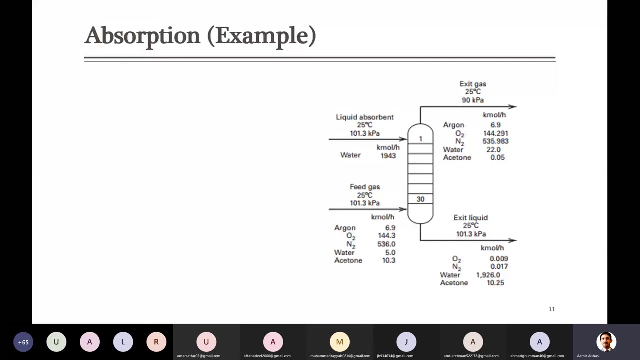 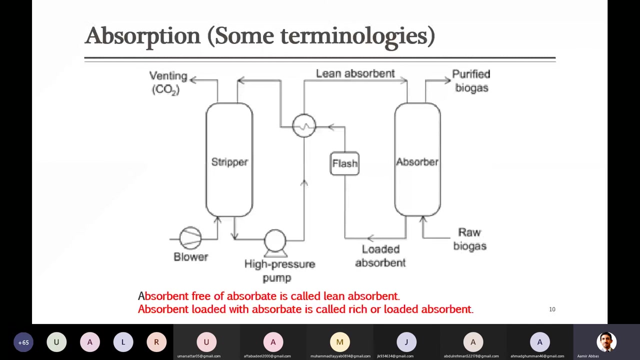 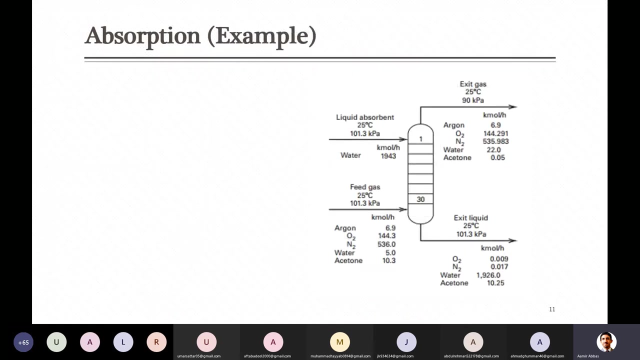 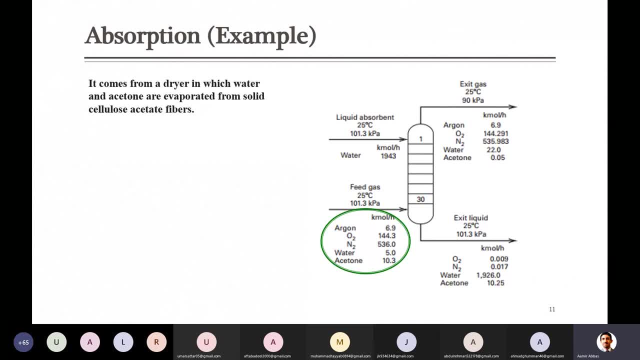 let's look at this, one of the other example, and that example is related to like air which is carrying somehow water and acetone, and from where it comes. i mean, as you can see in this diagram, this one which is highlighted part, this is the gas stream which is entering to some absorption. 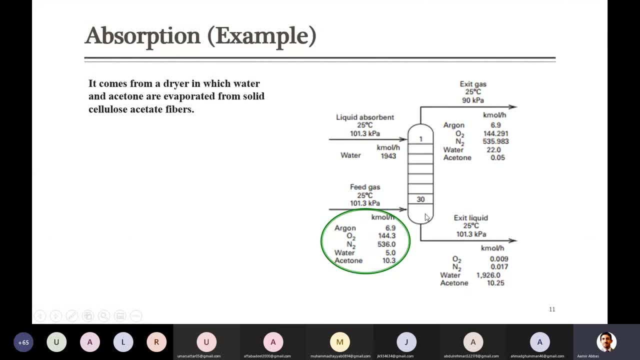 column. this is one absorption column in which there are 30 trays are installed. he has mentioned here 1 to 30 and in this case we- we are just starting with this- that feed gas is entering to this at room temperature and means one atmospheric pressure and that contains some five component. 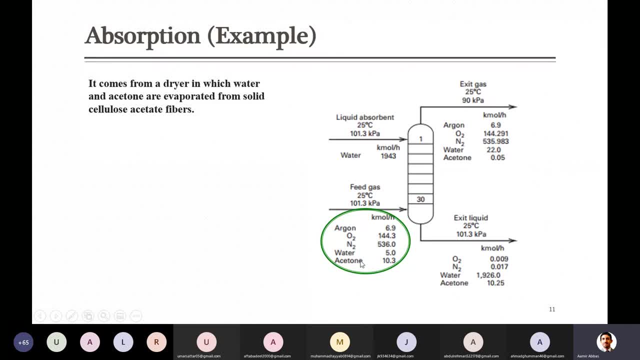 argon, oxygen, nitrogen, which are usually part of the air stream, but there is also water and acetone and he says that it comes from a dryer. dryer mean they keep and in which we dry some of the stream. so when we pass the air from that and maybe also we are- 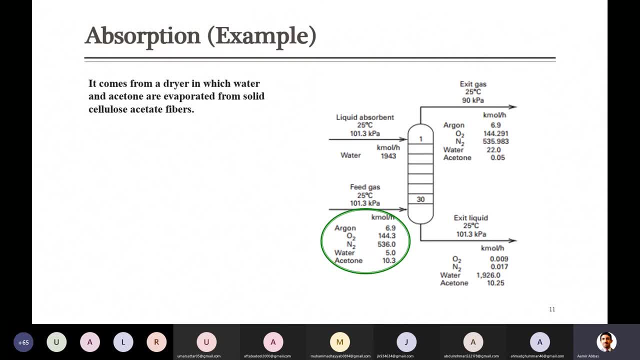 providing some heat so we can dry some stream. and i mean, during this drying operation the acetone and water are evaporated from solid cellulose acetate fibers so they become part of this air stream. so when they become part of this air stream, the purpose here is to regenerate the air so that 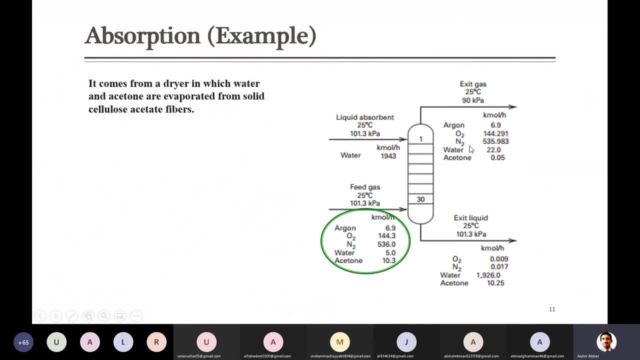 that can be again used for this process. so in this case, for removal of some of the components of the air, we are bringing in some liquid, and that liquid is liquid absorbent, and that is simple water. here, by the way, flow rates are given, i mean by your understanding. so the water here has the 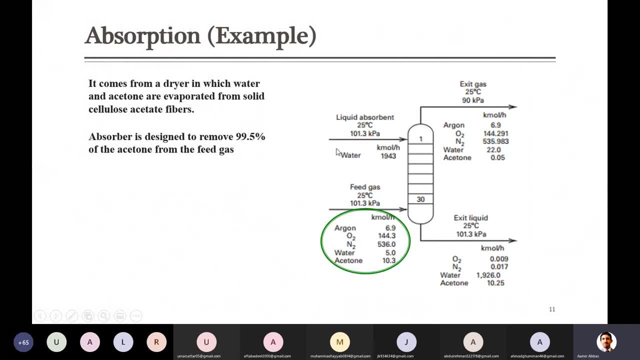 affinity that it can remove 99.5 percent acetone it is entering to this, which is, for example, here it is 10.3 kilo mole per hour. so out of this, 99.5 percent is removed and only 0.5 percent is just leaving with the exit case. uh so uh, when we are scrubbing. 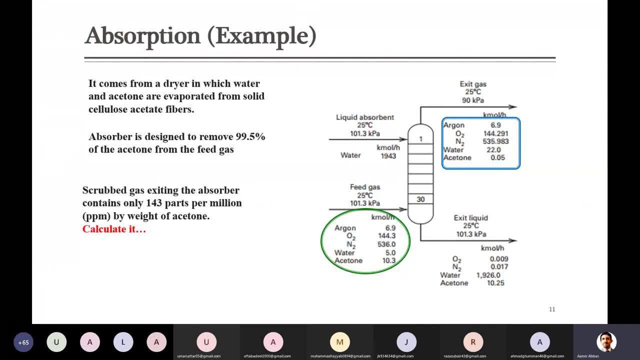 this gas i mean. usually scrubbing is like absorption and most of the time this terminology is used with scrubbing when you use water for the removal of some of the components. so here, because you are, we are using water as absorbent. so due to this, he said a scrubbed gas, the gas uh, which which has come, or 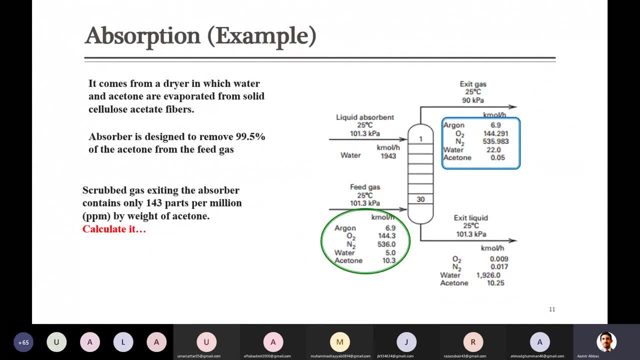 which came in contact with the water and uh, some of the species which were present in this has been removed and he said that the scrub gas exiting the absorber that contain only 143 parts per million by weight of acetone with this stream which is leaving from this, which were initially containing 10.3 kilo mole per hour. that contains 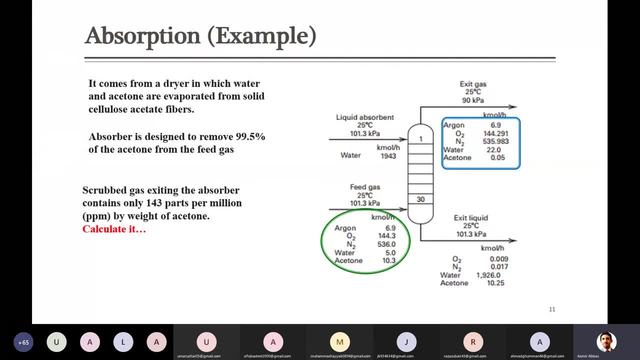 143 parts per million by weight of acetone. and, by the way, i have mentioned here that you have to calculate it. either it is, uh, exactly 130, 143 parts per million, or not. so, guys, i think you can do this calculation here. the moles are given, uh, this the basis data, the one hour. so all are like 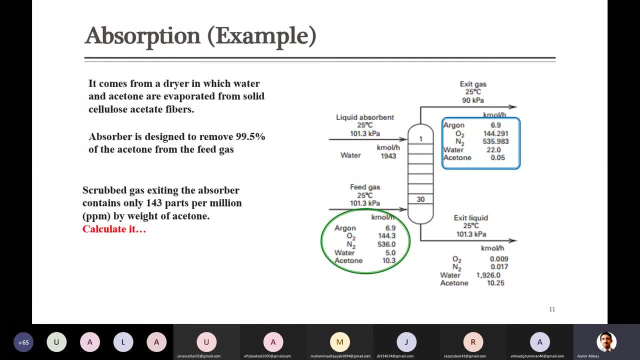 kilo moles and a few few days back we used the water in this tank so we can calculate the volume of the water. discuss this: that when there is a written something, ppm- and, as he mentioned here, that this is ppm based on the weight, so it means this is 143 gram per gram of all the species. 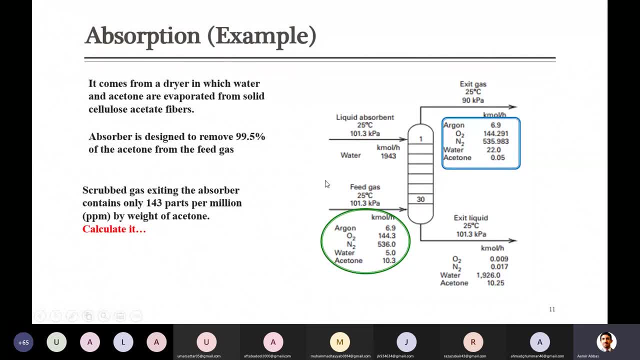 present in this gas. so in the division, and that is mean gram per 10 to the power, 6 gram of all the species. so just do this calculation. here the moles are given and you can convert. you know the components, so you can convert these moles to the amounts by multiplying with their molecular weight. 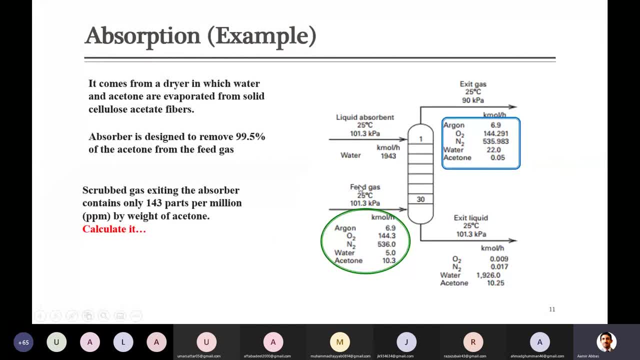 so i mean from that. then you can just do this calculation: either it is 143 parts per million or not. currently go for this. so here the water is. actually, if you look, the water is part of gas stream as well, as water is being used as an absorbent from the top. so here with the water, both phenomena takes place and 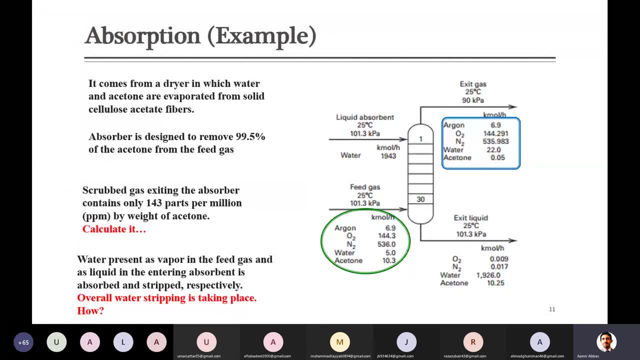 those phenomena are like, for water stripping as well as absorption of the water will be taking place. the water which is part of the feed gas, this water molecule, or these water molecule, are actually absorbed inside the liquid stream. there is water as well, so acetone and water. 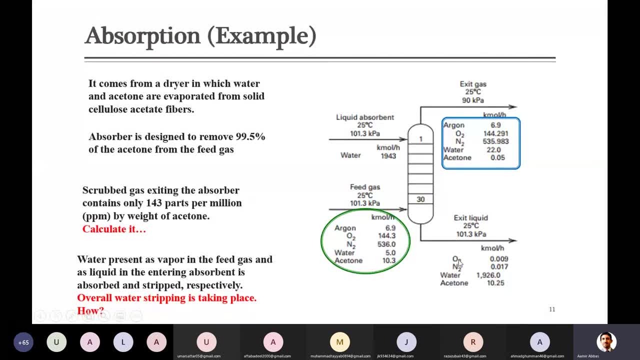 are actually absorbed here, mainly along with the some of the water which is being used as an absorbent from the top. so here with the water, both phenomena are actually absorbed inside the liquid stream. there is water as well as absorption of the water, which is amount of. you can see that oxygen and nitrogen. they are also removed in some small amount. but 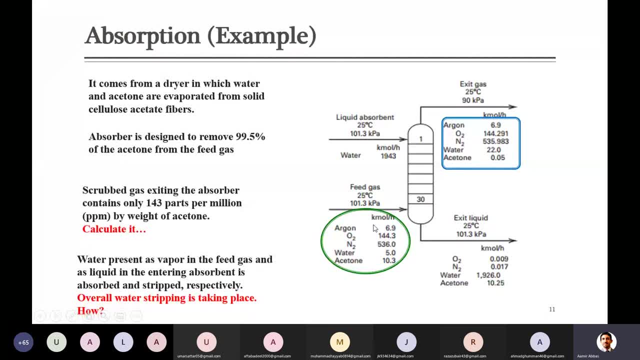 most of there is going to the top. so at the same time when water is coming here, some of the water will be stripped with this gas and if you look at this, the water amount in the stream which is leaving at the top is 22 kilo mole per hour and when it was entering to the column it was only 5. 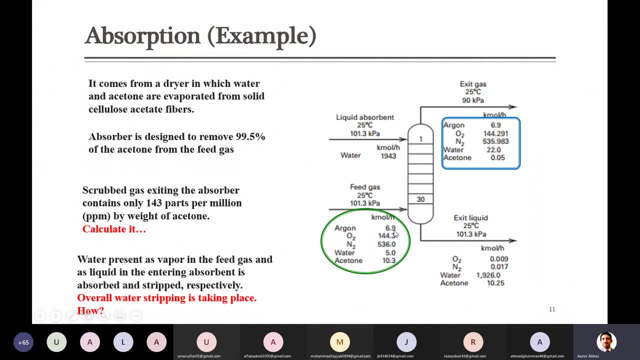 kilo mole per hour. so it's mean overall, instead of absorption, the stripping of water molecule has taken place. the gas has taken away the water molecule with this, so here in major absorption of acetone, along with some nitrogen and oxygen. by the way, why water has gone with this air? can anyone tell me? 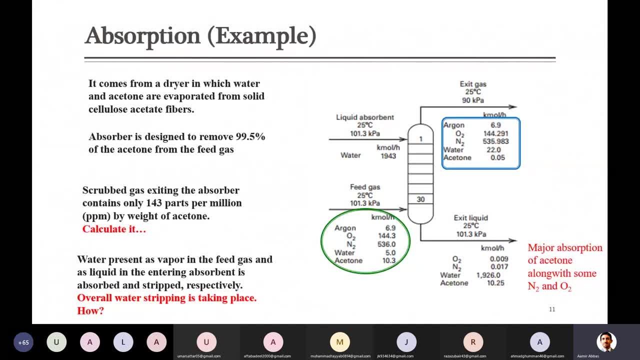 guys, do you know that air has the affinity to carry water molecules? always they are in our surrounding that contains water in sufficient amount. so here, when air was coming in contact and that that was carrying some small amount of the water, and if air at the given temperature and 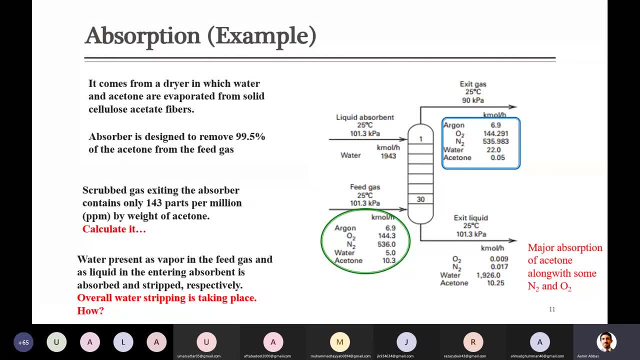 pressure can carry more water molecules, so that will just take water from this stream and they will carry water molecules with this. so the reason is this: that air can carry more water and if water is in less amount as compared to the maximum which air can carry at, 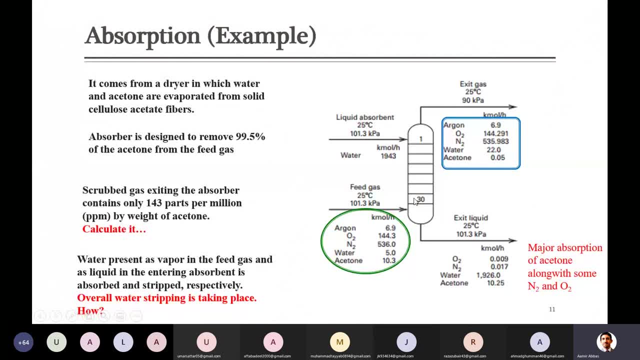 the given temperature and pressure. so when water will come in contact with this, definitely it will carry water with it. so that here two things are important, which i discussed in last slide: that always, when there is, for example, anything which you want to remove, not 100 percent remove, 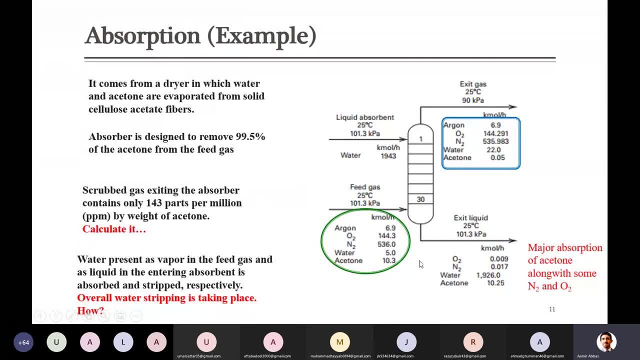 as he mentioned, that 99.5 percent of acetone is removed technically. at the same time, the thing which, when you are absorbing from the gas, it is not only the one component which is completely, i guess, which you want to remove that should be absorbed, but other components present in the gas. they are also absorbed in. 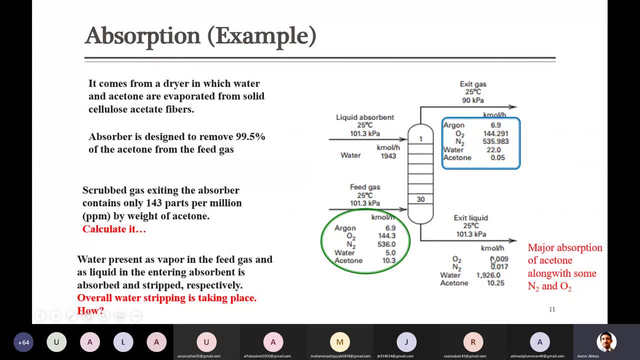 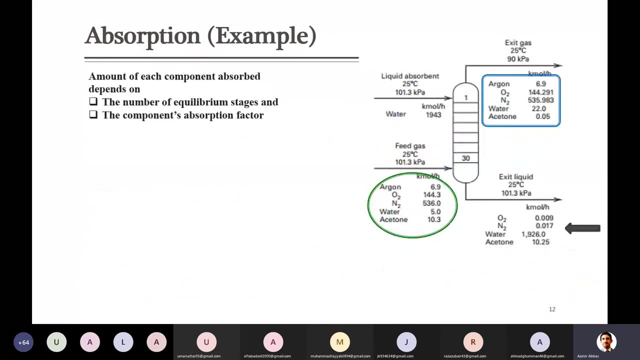 small amounts, for example here oxygen and nitrogen. you can see so in all of the processes which we see in like industries, there will always be some small amount of these. other components will also be going or absorbed. so why it happens are on which actually parameter it depends. so amount of each component which is absorbed, it depends on two major components. 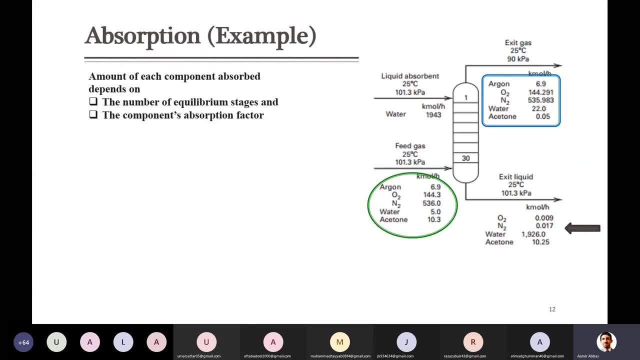 which are like number of equilibrium stages, uh, whenever there will be large number of stages, definitely absorption will be higher and at the same time, the components, absorption factor or assumption factor are. so how we define at in front of this, define it these which uh any of the component of the gas, its absorption factor, and what is absorption factor, or how we 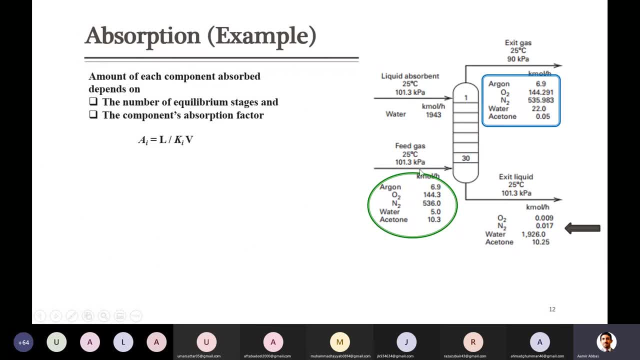 define it, that absorption factor is actually equal to uh. this is liquid flow rate divided by k, uh equilibrium constant. and then there is why in this vapor flow rate- v for vapor and and for the state payo and gas flow rate and uh- it also depends on the uh kilogram constant. so this k value, how you? 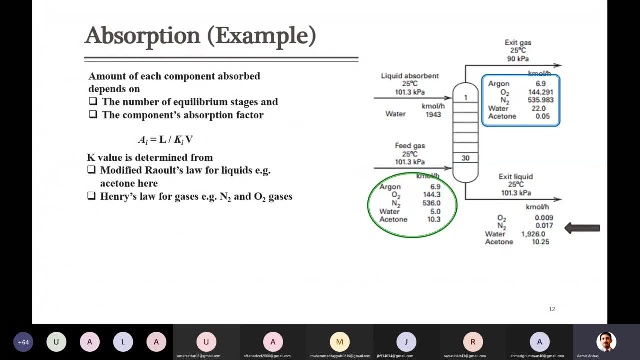 determine, uh, that k value. i think these things you have studied in thermodynamics as well as, hopefully, in life. the course, which was fundamental, do you guys already know, studied this. anyone answer this please? k value determination, yes, so, okay. so, uh, due to this here, uh, if, if you don't remember, or 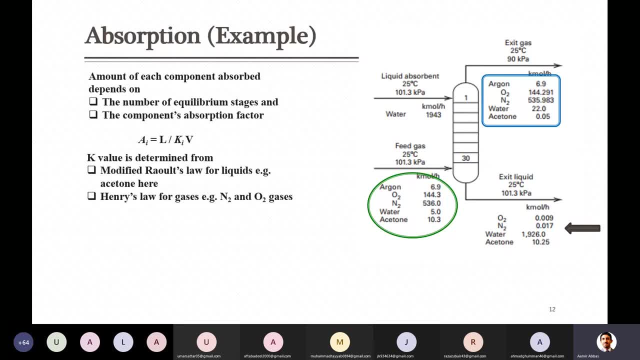 you don't know, in the book it is mentioned that in the chapter two there is a complete chapter on this and you are supposed to like study this before coming to this course in thermodynamics as well as in the fundamental course. so if you don't remember, kindly just quickly go through. 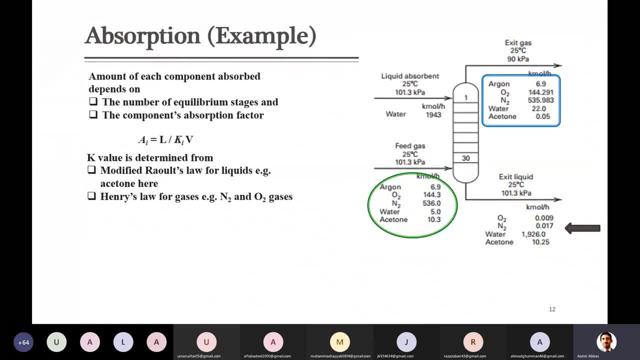 the chapter two. uh, he mentioned something specific table in this chapter six. uh, this is actually chapter six, so i just note down from there. and uh, he mentioned some specific section in the chapter two. you can go there and revise it. but just here, quickly for your information: k value, uh, for light liquids, that we determine with the 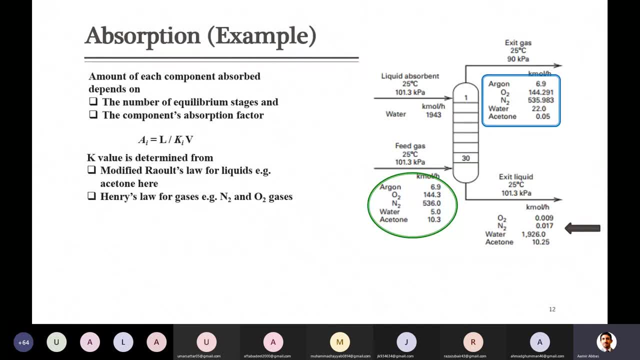 help of routh's law and hopefully you know its main equation. so, uh, sometimes, if the concentrations are very low, the amounts are very low. then modified route slides used for this determination of k value, while for the gases, for example? here the gases are nitrogen and oxygen and argon. so 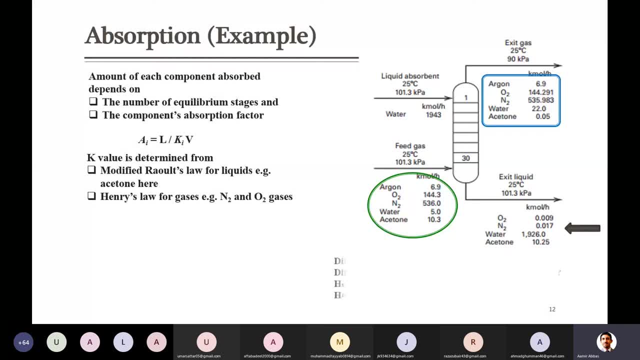 in that case you usually use henry law for the determination of these k values. so here are. there are few questions for you. i mean, uh mentioned here below the diagram that what is difference between ideal and non-ideal solution. you should know, if you don't know just. 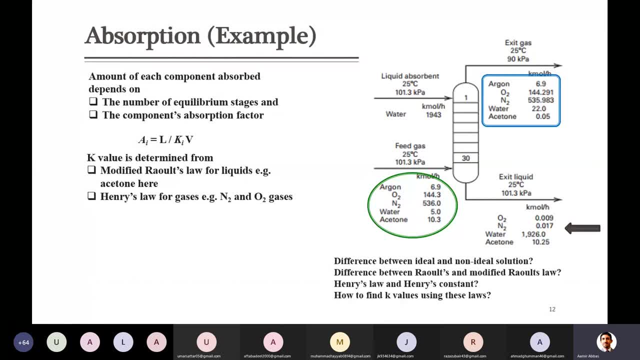 try to search the answer. this is your like small homework again, and just just note down the answers with you and maybe next vector, i will quickly discuss this. so what is difference between, like routh's law and modified routh's law as well, henry law? what is henry constant? so, and then how to find. 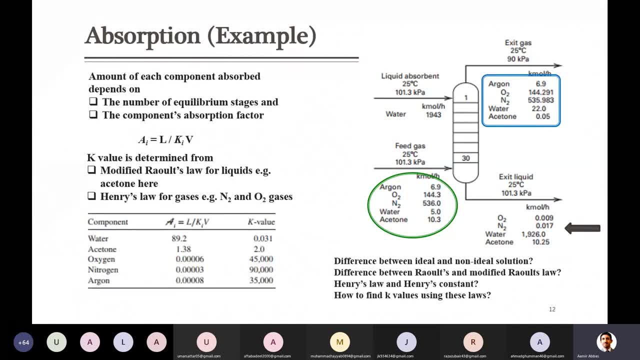 k values using these laws. actually, when you know the equation, definitely you can find the k value, but before that we should know what are the equation of these laws. so that's what we are going to do, is we are going to use the routh's laws and in what cases they will be used. so here for the 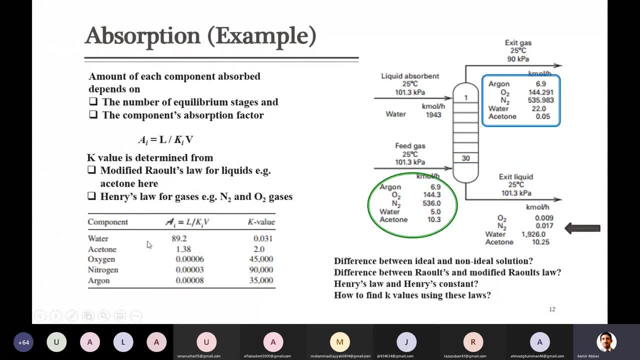 components which were available in our test stream which was entering to the column. they were argon, water, acetone, nitrogen and oxygen. out of these, for water the routh's law is used and for the other component, like acetone, which is also a liquid. so for that i mean at normal room temperature and 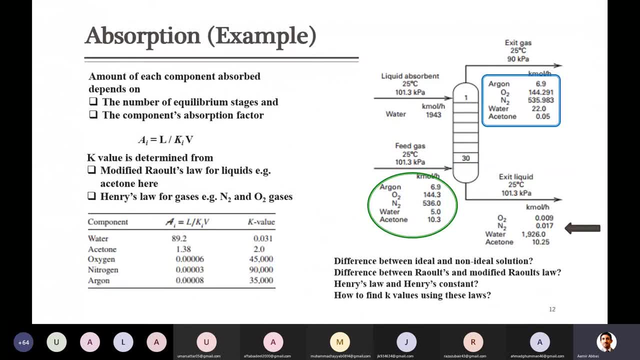 pressure, it is a liquid. due to this, i'm saying it is a liquid. so this is determined with the help of modified routh's law. due to the very small amount- low amount as compared to the overall- its concentration is small. so whenever we are determined- it's like k value and then absorption coefficient- we will be using modified routh's law. 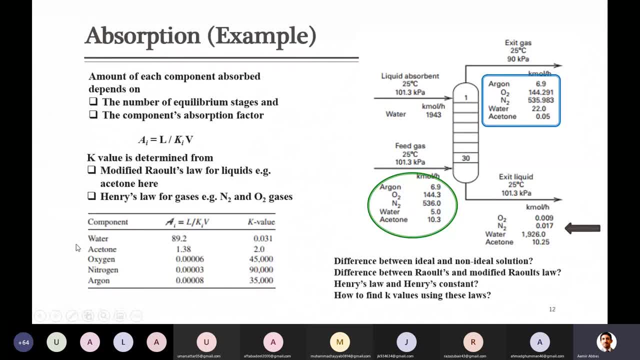 and for oxygen and hydrogen and argon, the mean henry law will be used. so, for an economic prospect, the value of a, this absorption that should be in the range of 1.25 to 2 for any of the components when you are looking for this. 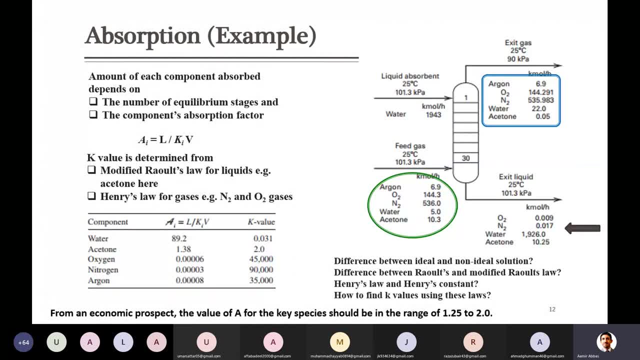 a, for example, we have to decide the a, so a: first of all you determine the k value and then you have determined the k value. that then you go for like liquid and while vapor flow rate and this value should lie in this range, mean, as we mentioned, for economic prospects. so i mean for. 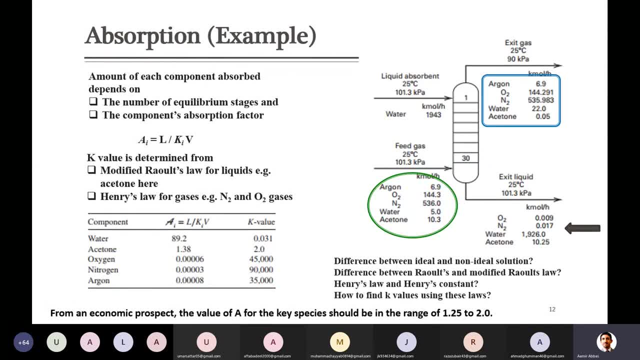 economically to run this plant or this process. if this value is lower than this, definitely this process will not be suitable. in that case, either you have to increase the mean some flow rate or decrease some other flow rate, or maybe you have to switch the liquid that can give you better k value. 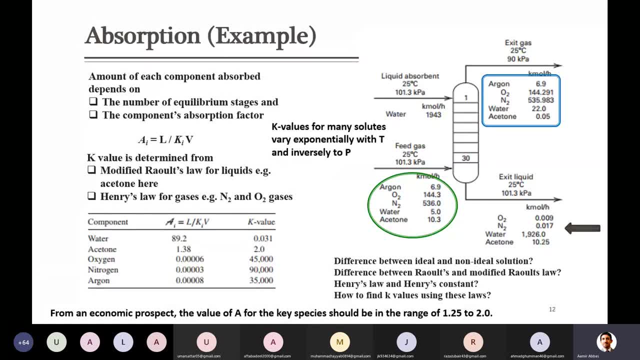 so this k value for many solutes vary exponentially with temperature and inversely to the pressure. so if you remember this routh's law, that is something p set over p. is that the equation for routh's law? yes, this is, and if it is modified routh's law, then some some coefficient comes with this and p. 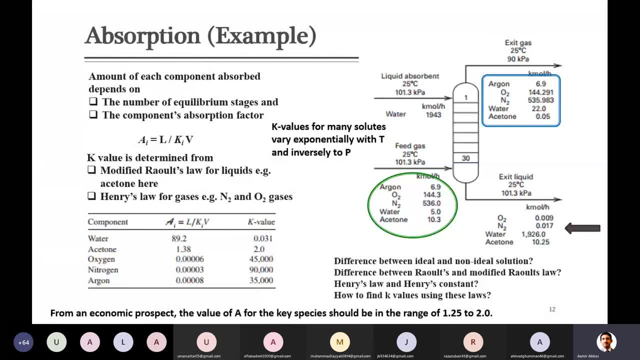 set over p. so in those cases, if you just look at the value now, as i mentioned that the equation is for henry, for example, for routh's law, we consider that it is p set over p divided by p. now if you increase the pressure, so what will happen? the value of k will decrease because that is equal. 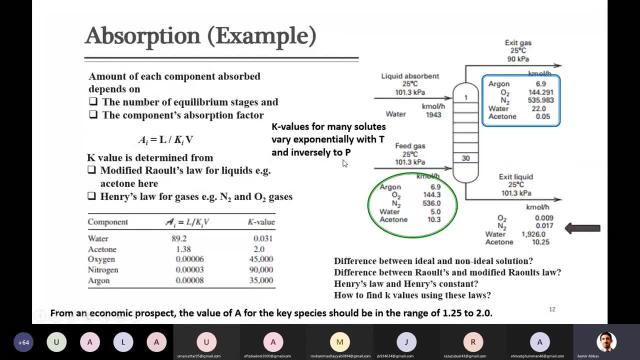 to k is equal to p set over p. so in that case, when you increase the pressure, so due to increase in this pressure, the value of k will be decreasing. so when the value of k will be decreasing, look here in this equation this is in denominator k and v. actually, so when you reduce the value of k, 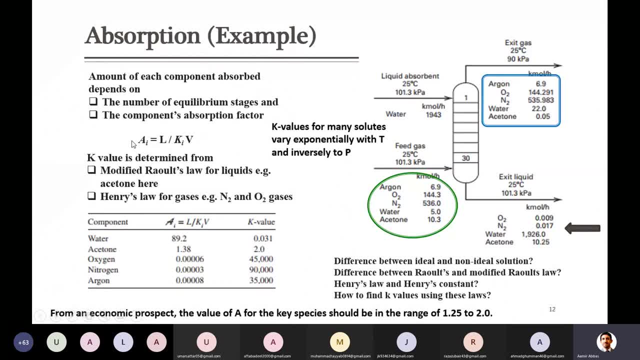 what will happen to the a absorption factor? it will increase, definitely it will increase. so just link it again. the first point i said: when you increase the pressure, the value of k is decreasing, and when value of k is decreasing, absorption factor is increasing. it means absorption will be increasing. because here we said, absorption is like 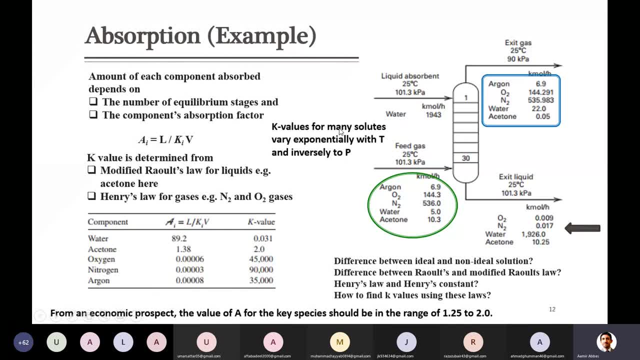 dependent on these two. so you know that in case of absorption, high pressure will increase the value of favor, the absorption okay. so high pressure mean like when you will be like increasing the pressure, definitely that actually increase here this absorption factor, and i mean that that helps you. 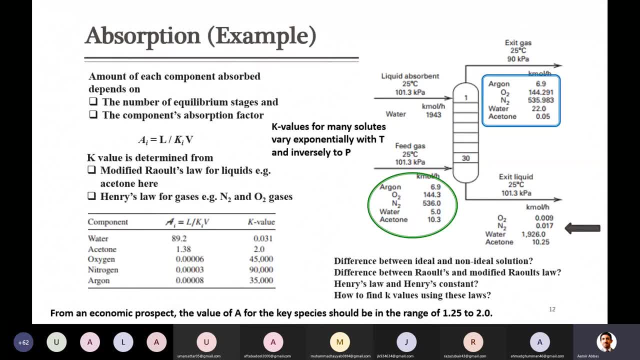 so in case of like he mentioned, as here, like with the temperature, it it increases, raises mean value of k will increase with the temperature. so when we increase the temperature value of k is increasing. and when value of k is increasing here the absorption factor is decreasing and due to that 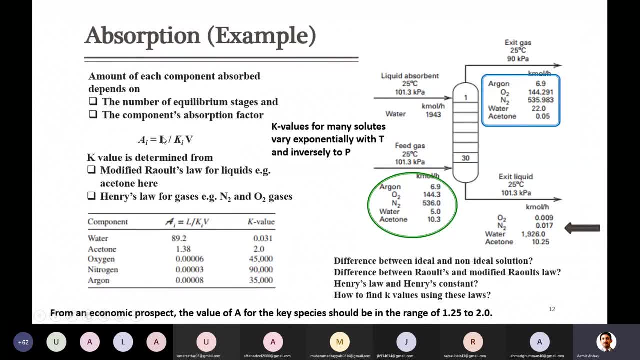 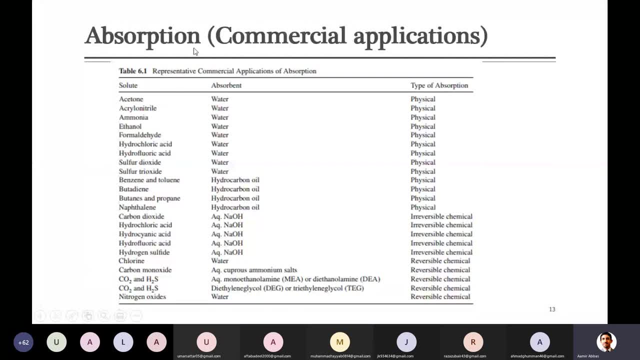 your absorption amount will decrease in that case. so that's it, i think. okay, i will just stop here, finish it here. so, absorption, commercial application- uh, here in this table are mentioned some cellulose. cellulose mean those species which you want to absorb from the gas stream. 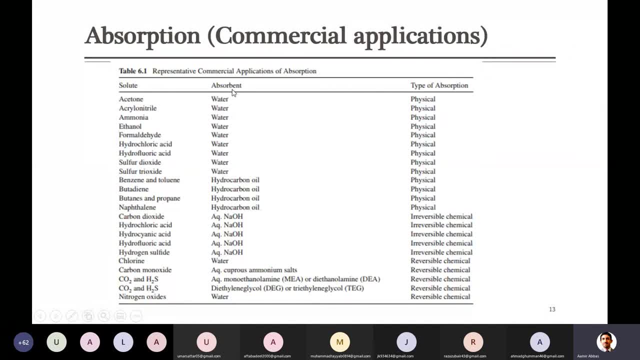 and other are the absorbent, the liquid, the solvent, which are used for this purpose. and then mentioned is the type of absorption, uh. so out of these here i will just directly go to those which are considered more favorable. they are like reversible chemicals. so for carbon monoxides, are this carbon dioxide, h2s removal? you can see that these monoethanol amine 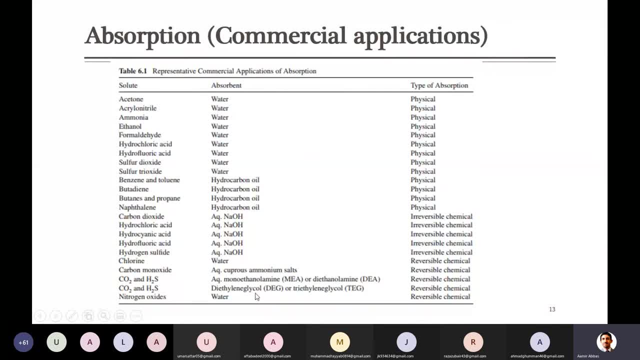 and diethanol amine are used. sometimes glycols are also used in this diethyl glycol dry head in, for example, here he mentioned, for nitrogen oxide water is used and that can react this. so out of- i mean various are now i mean out of these- all various examples, given they are used actually on. 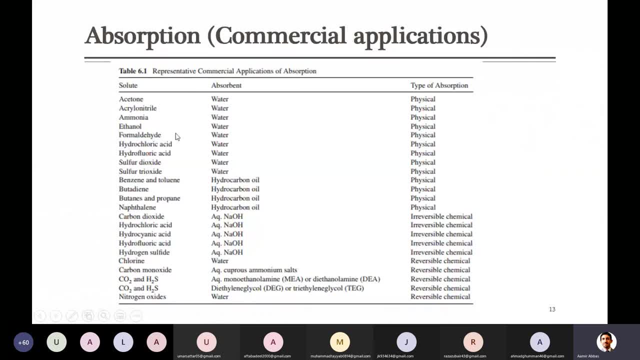 industrial scale for removal of the component which are mentioned here, and these are the solvent, by the way. uh, when, whenever you have to select, although chemical is better, but in some cases maybe there is a little bit of a difference between the two, so that's why it's important to 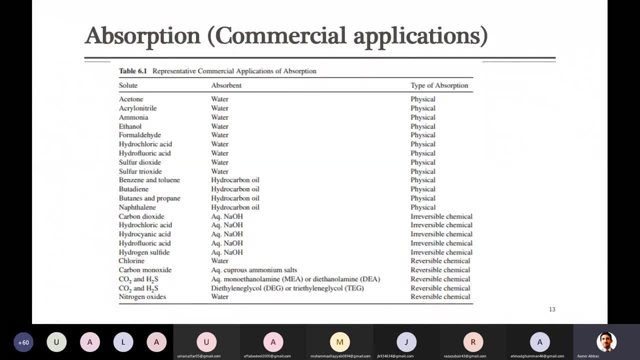 make sure that when you are using the solvent, you are using it in the right way. so that's why it's important to make sure that when you are using the solvent, you are using it in the right way. so in those cases, uh, then definitely we have to use that, although absorption will be low, as 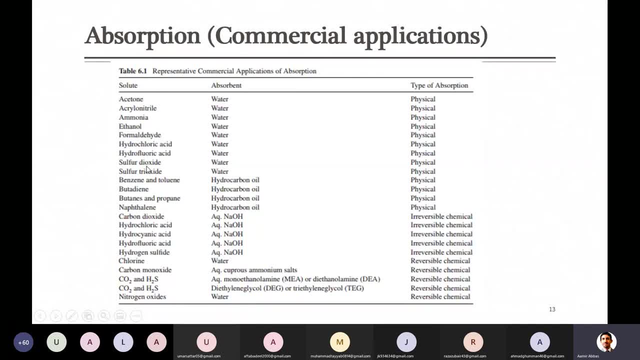 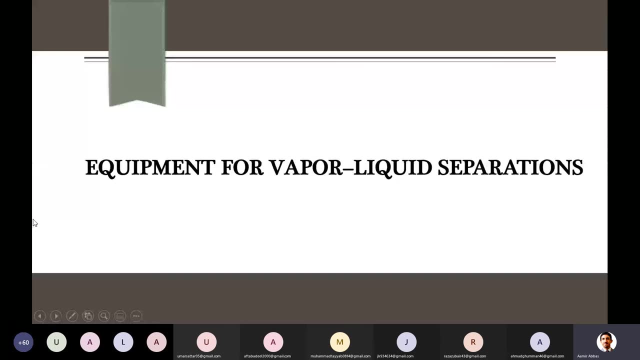 compared to the chemical, and you will need huge equipment, maybe more number of stages, but in case of chemical, i mean, if you can have that option that is more preferred and, in chemical, reversible already, as we have talked about this. so next, uh, although i was supposed to start this today, but okay, fine, tomorrow we will start with this. 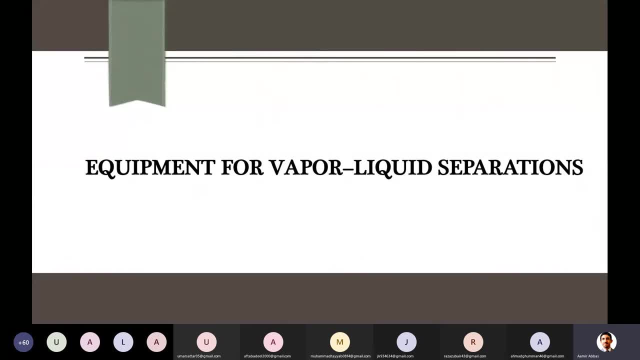 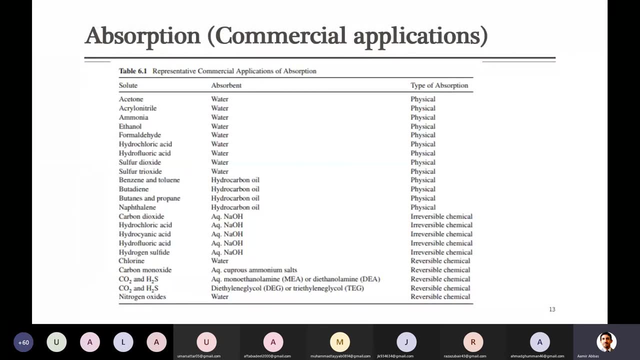 equipment for vapor liquid separation and initially with the, we will be introduced with their internal mean, the structure of the equipments quickly, i think in next few lecture, uh, hopefully we will be able to cover the equipments which are packed tower as well as, like great our, their types of tower, types of packing and so on. uh, which one is better? and i mean their.